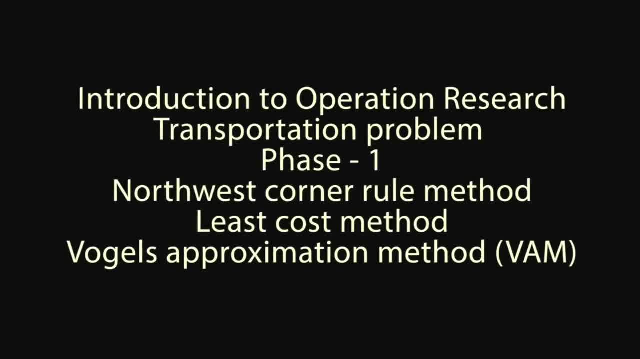 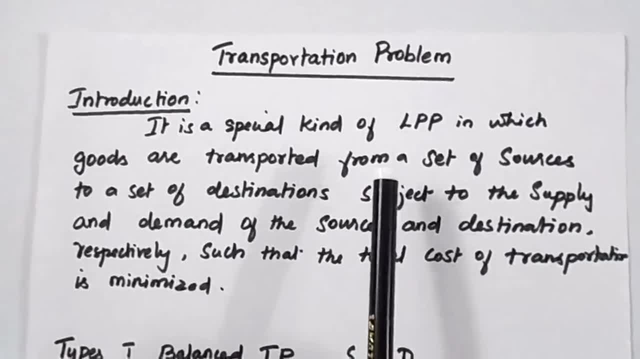 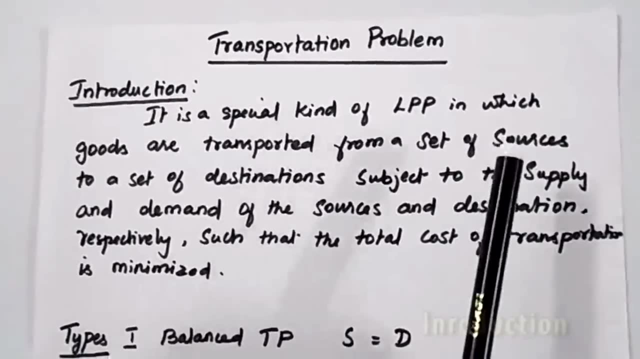 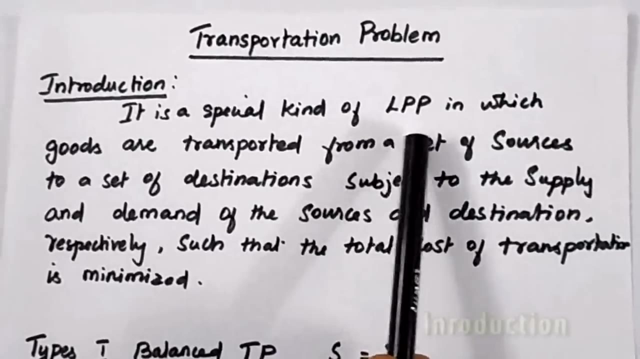 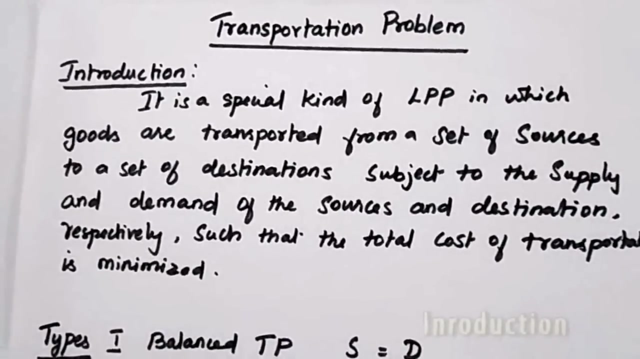 Hi, in this video I am going to explain transportation problem. So before I am going to explain how to solve the transportation problem, let me explain introduction about transportation problem. Transportation problem means it is a special kind of linear programming problem in which goods are transported from a set of sources to set of destination, subject to 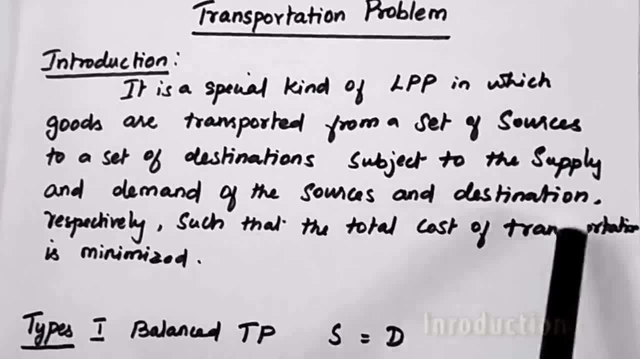 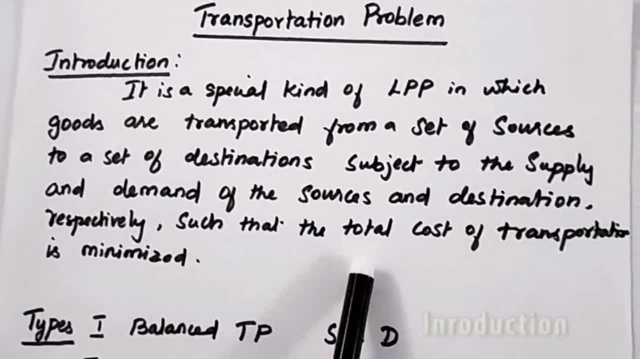 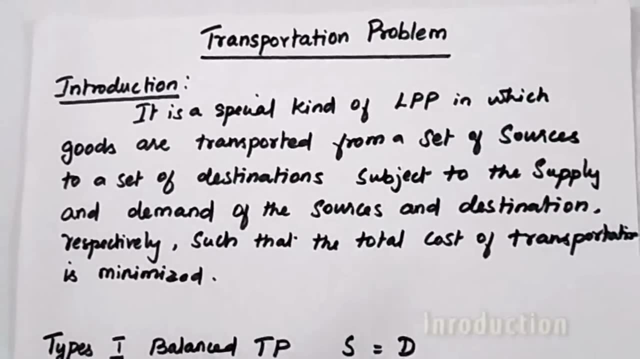 or according to supply and demand, of the sources and destination respectively, such that the total cost of transportation is minimized. The ultimate objective of this particular technique is: in order to reduce the transportation cost, we need to apply some technique So, with the help of this, we can able to minimize or identify the method in order to reduce the. 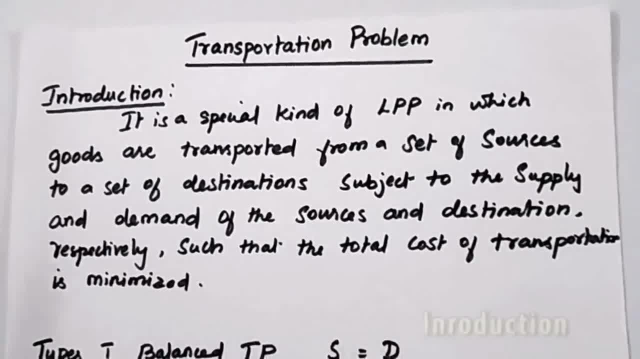 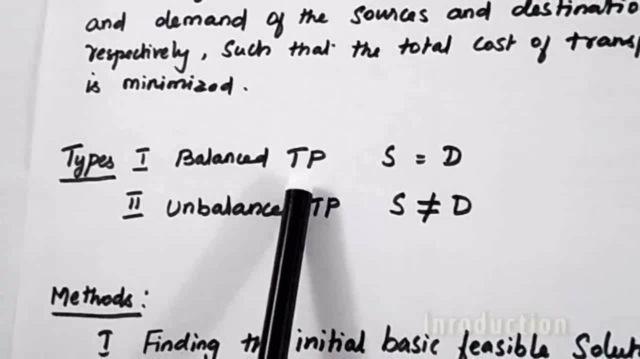 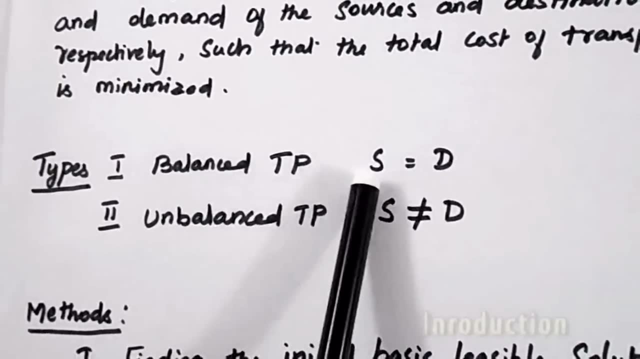 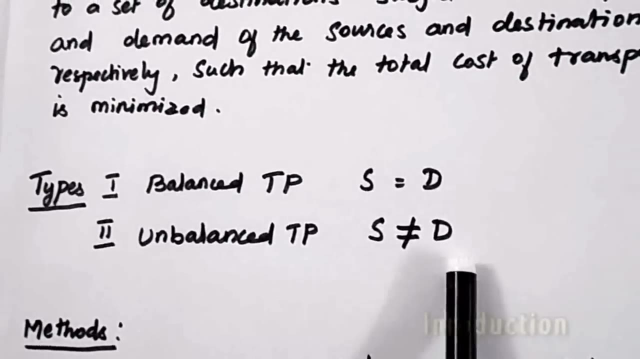 cost. Let me explain two different types of transportation problem. First one is balanced transportation problem. Balanced transportation problem means both supply and demand will be equal. Then it is called as balanced transportation problem. Unbalanced transportation problem means supply is not equal to demand. It means unbalanced transportation problem. We cannot. 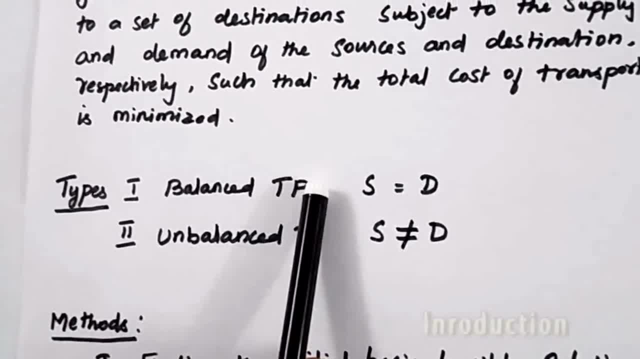 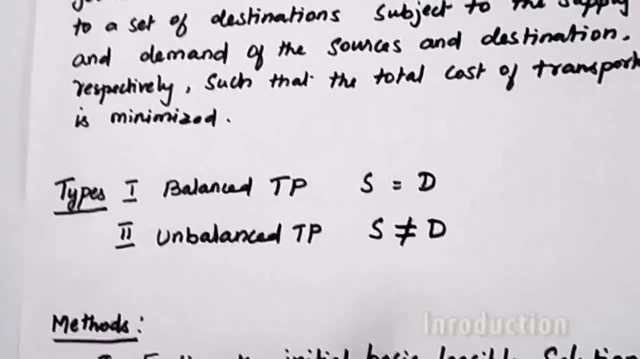 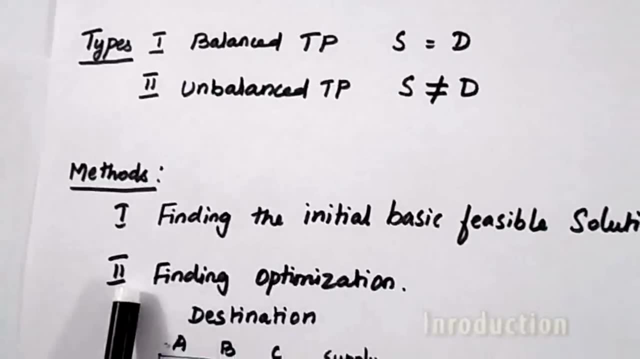 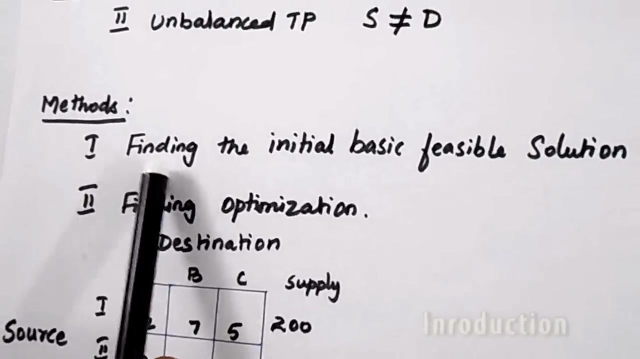 with unbalanced transportation problem. to balance transportation problem we need to add either dummy column or dummy row, according to the situation. so there are two types: balance as well as unbalanced transportation problem. then methods of transportation problem. generally there are two phases for transportation problem. first one is finding the initial feasible solution. 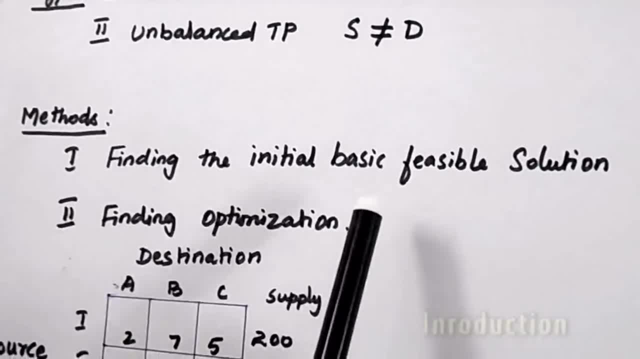 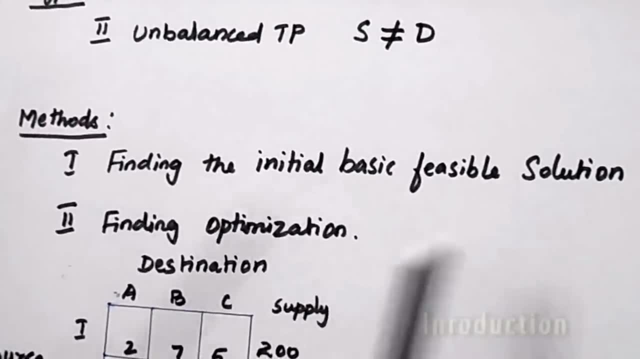 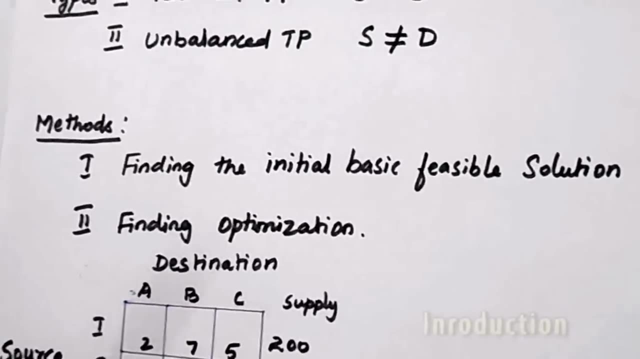 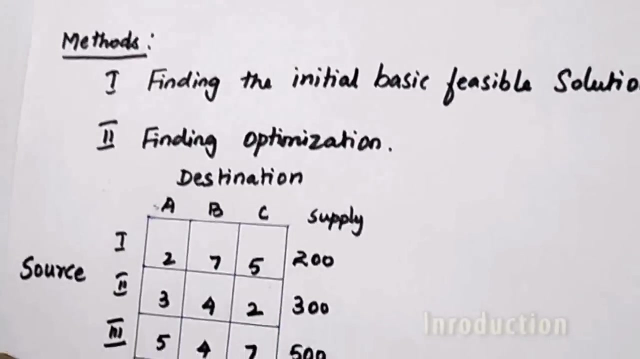 that is the first two phase. first we need to identify or find initial feasible solution. after finding this, only we can able to check the optimality, which one is best optimum. optimum means the maximum and finding the best among the various alternatives. that is second phases. so now I'm going to explain with the 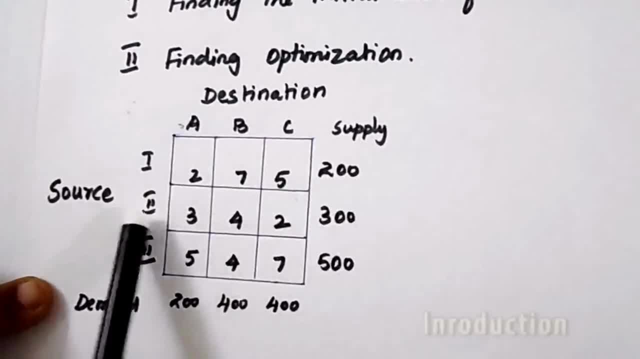 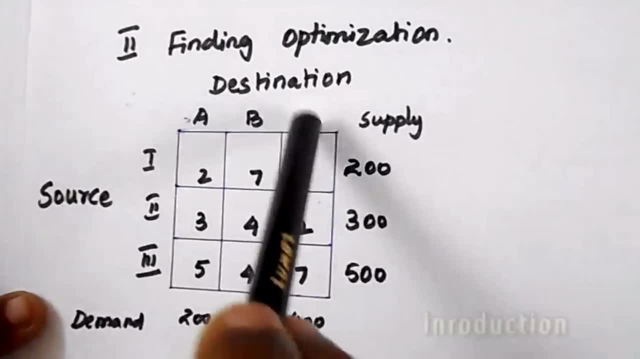 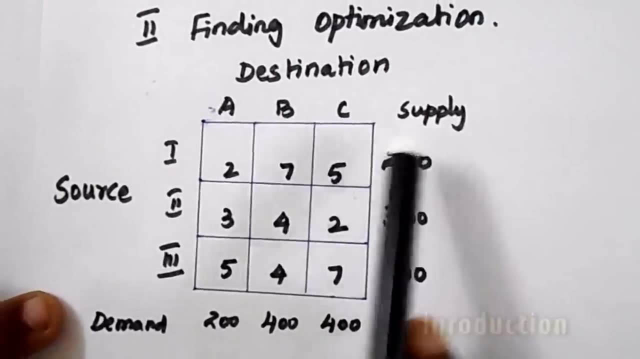 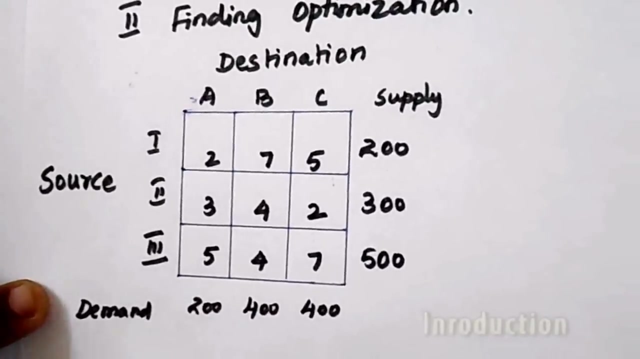 example. so this is called as row: first row. second row, third row, row. these are the three sources are available, okay, a, b, c, three columns, each sources and each row. you'll have some supply in each column. you'll have some demand. i told you no balanced transportation problem. before you proceed, just see or confirm whether it is balanced transportation. 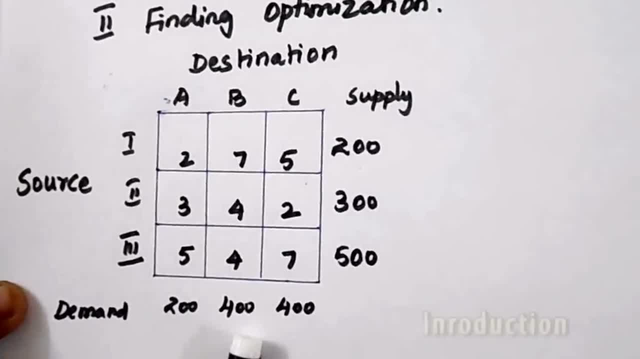 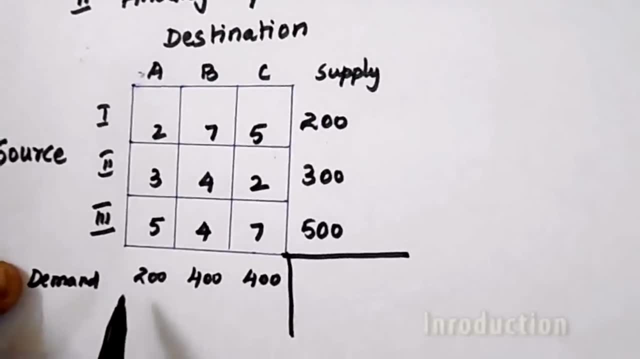 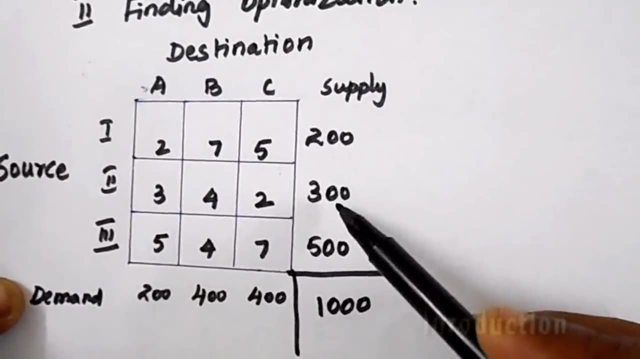 problem or unbalanced transportation problem. how can you find out this? just compare the demand and supply according to this problem. just see the demand: 200 plus 400 plus 400 000. just see the supply: 200 plus 300, 500 plus 500 000. it is a balanced transportation problem with this problem. 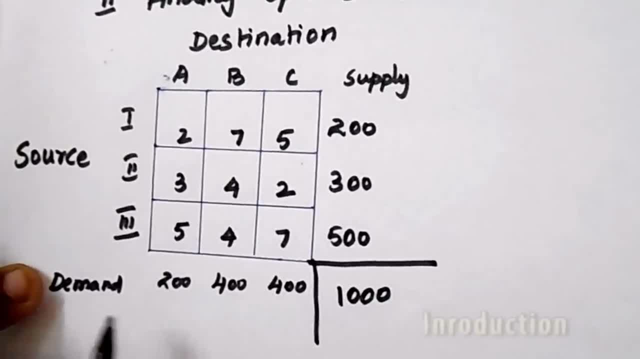 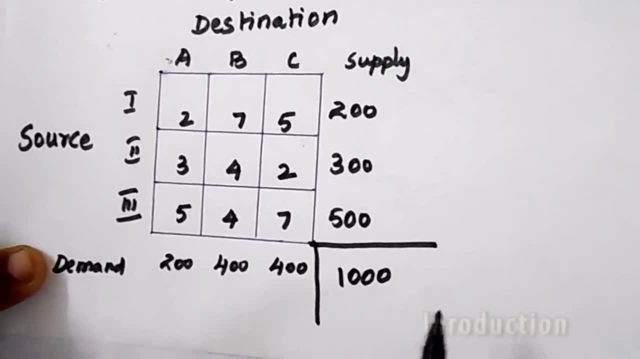 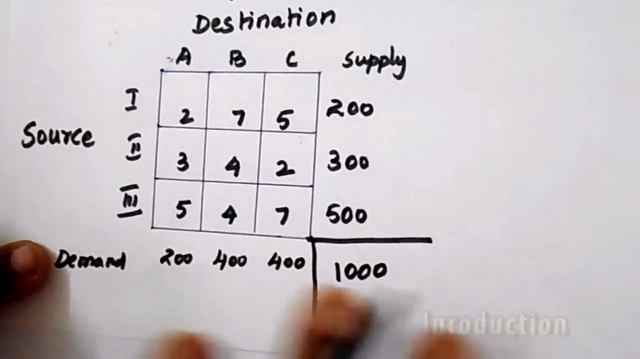 you can proceed. if it is unbalanced means demand will not equal to supply. what will happen in that case? we need to add one more row or one more dummy column according to demand and supply. but anyway, if you want to continue, the problem you need to have. 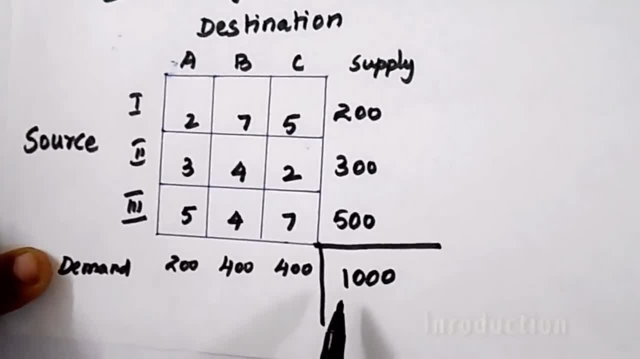 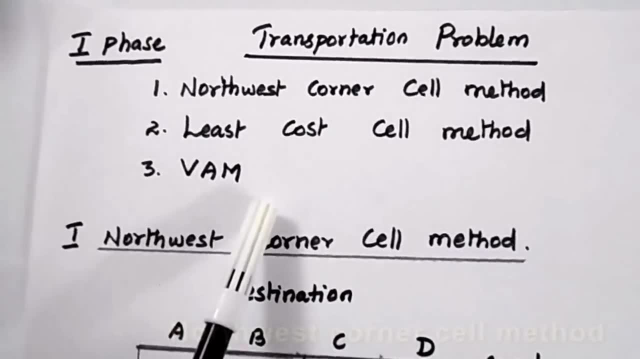 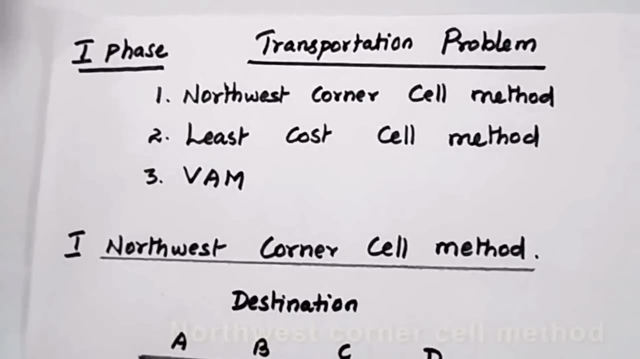 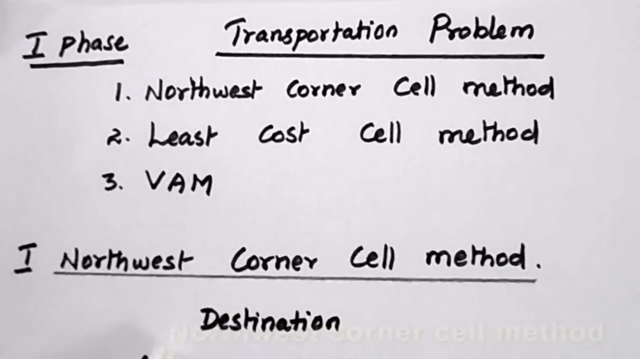 balance. balance means both demand and supply should be equal. let us see the three different methods of three different techniques to find the initial basic feasible solution. in phase one i told you no, there are two method of methods of solving transportation problem. so first phase is solution. after finding this, only we can able to check optimality. so according to check the initial, 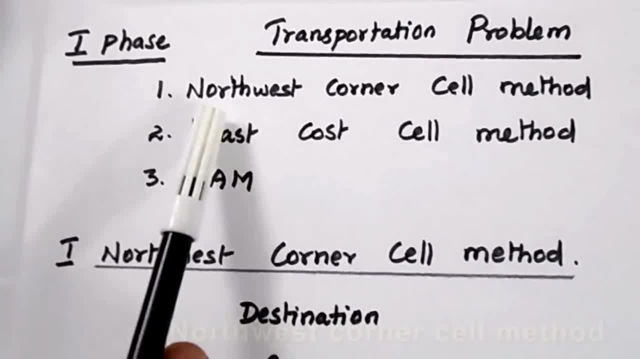 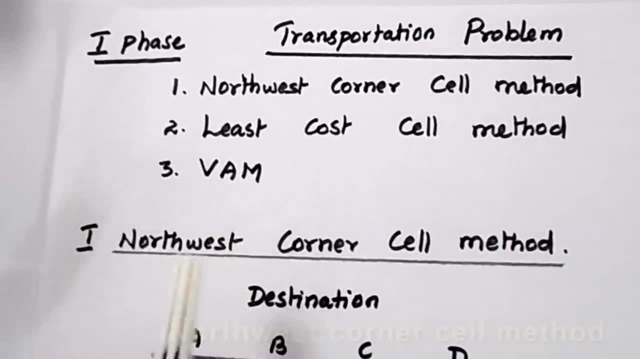 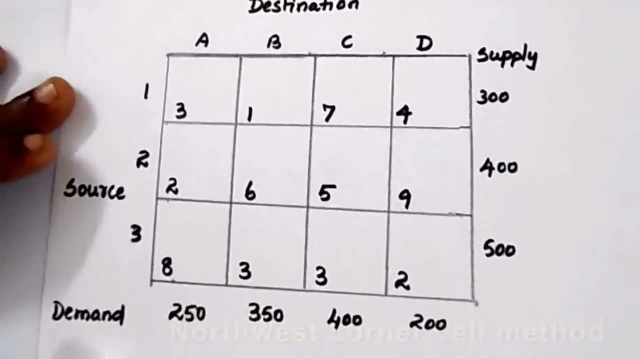 basic feasible. there are. three methods are available. first one is northwest corner cell method, second one least cost cell method and third one vam method. let me explain each and every one clearly. first one is northwest corner cell method. so this is a transportation problem we'll have. 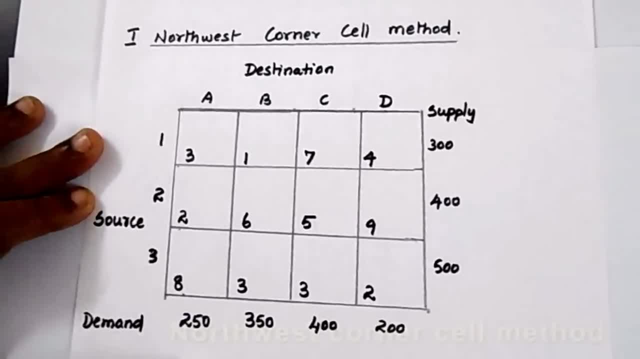 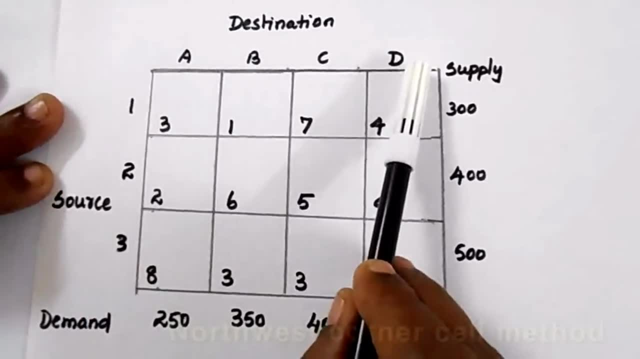 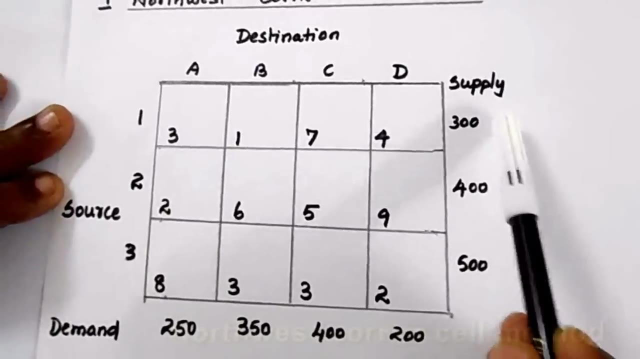 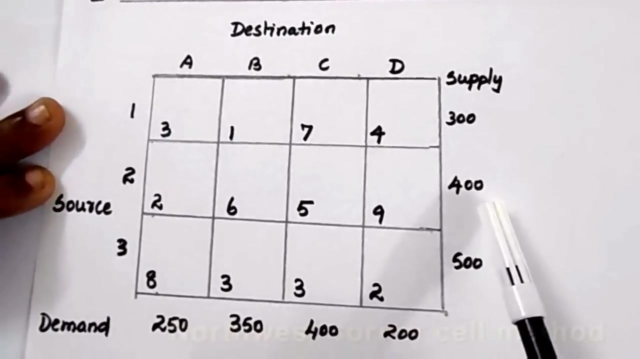 different sources and different destination. so according to this problem, there are three sources are available- sources one, two and three. and four destinations are there: a, b, c, d. in each sources and each destination some value is given. this is called as supply for source one: 300 supplies are available here. 400 supplies are available. 500 supplies are available. 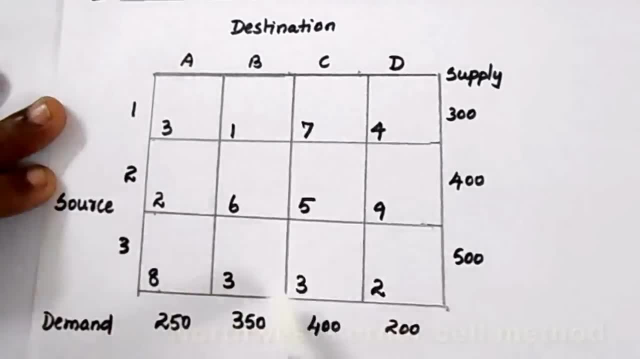 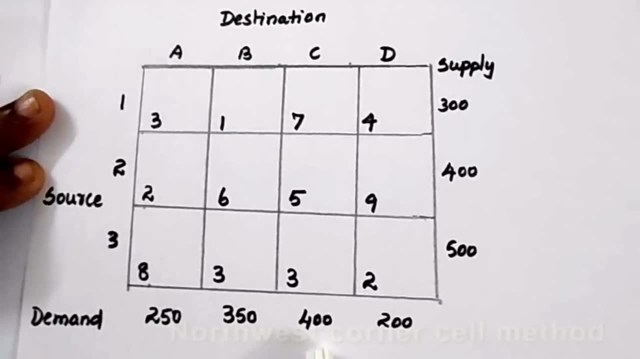 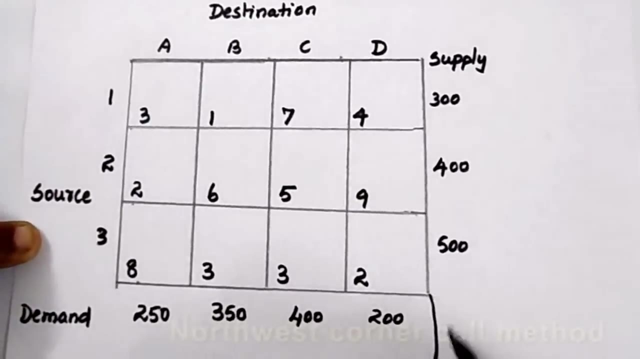 for each destination. this is column no for each destination. we have some demand for a: 50. demand is there for b: 350, for c: 400, 40, 200. before you solve this problem, first we need to check whether the problem is balanced or unbalanced. balance means both demand and supply will be. 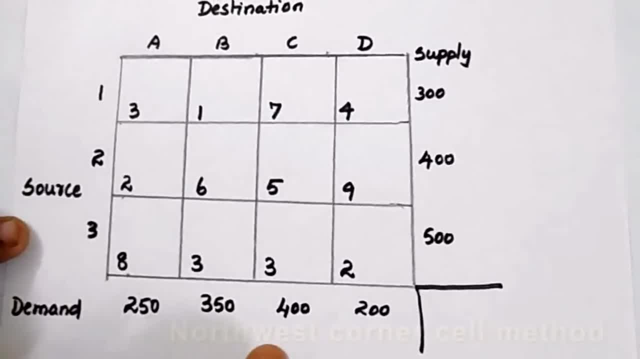 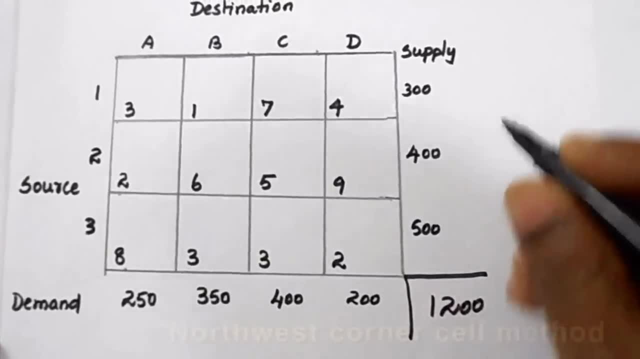 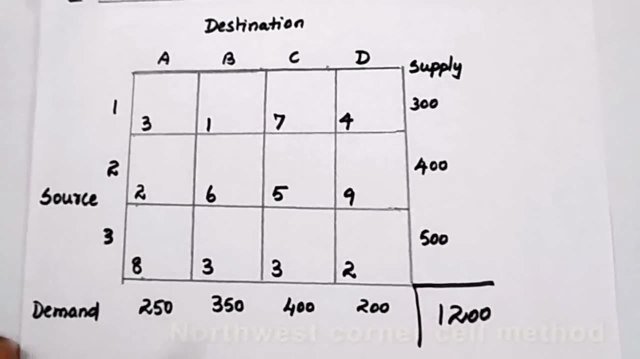 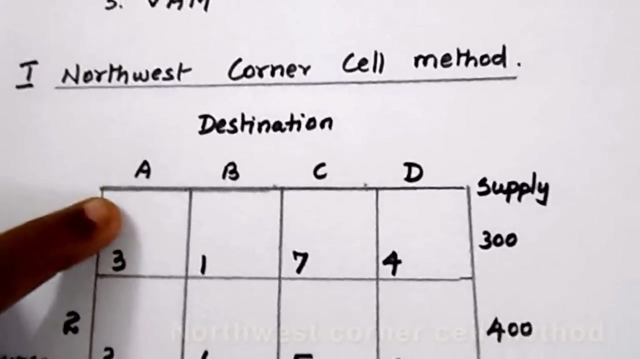 equal. just check 250, 350, 400, 200. what is the total thousand? 200. just check the supply: 300 plus 500, 1200. so it is a balanced problem. now we can proceed. so, according to northwest corner cell method, you have to start with this corner. this is a northwest corner, so you have to start with. 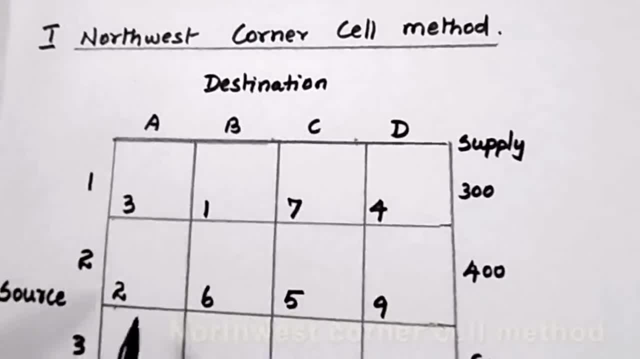 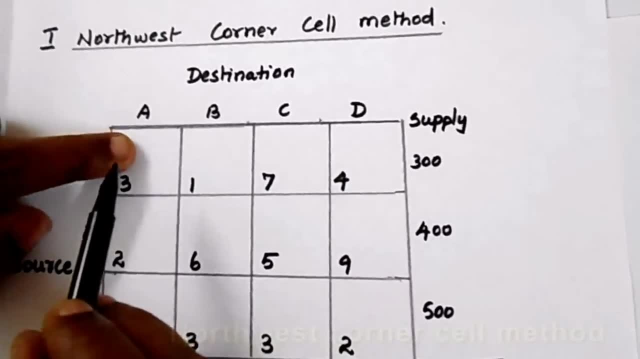 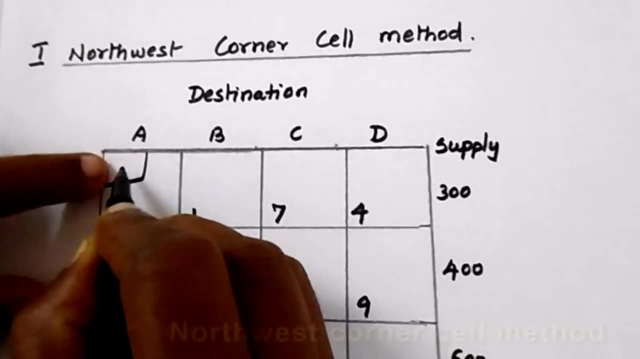 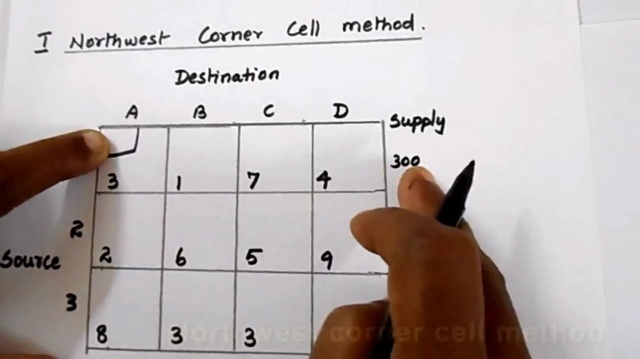 this cell, each and every element of this cell is considered as a cost per transportation. so first you have to start from this cell. this is the northwest corner. you have to start from here, just allocate. before you allocate the value, you have to compare demand for the particular column and supply for the particular row. here. 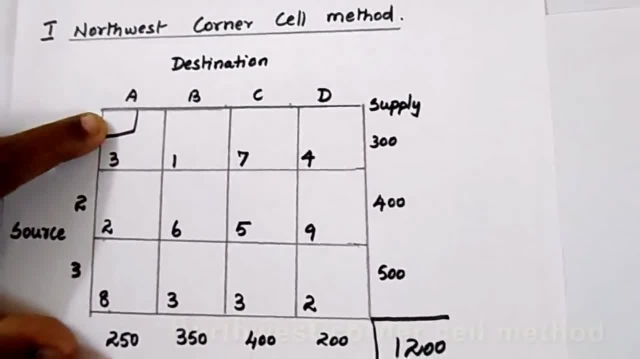 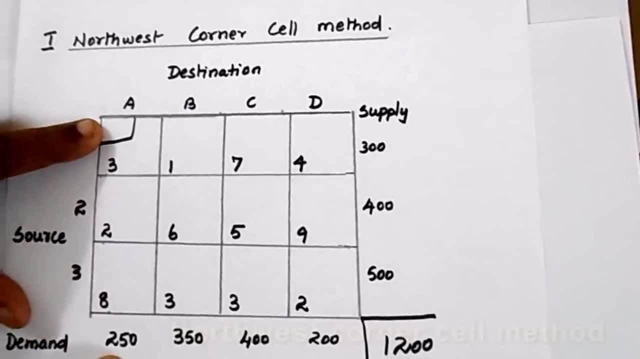 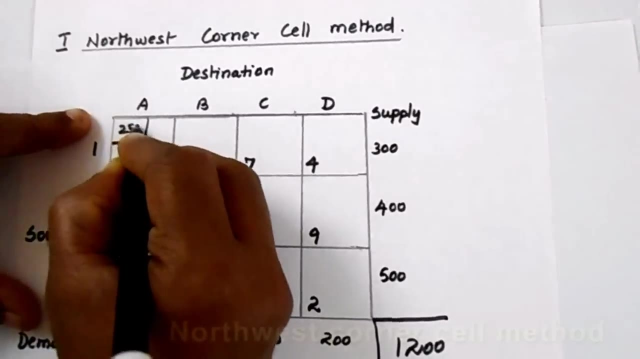 supply 300, but demand is only 250. so which one is lesser value? demand is less, so you have to allocate only demand because demand is lesser than the supply. so based on the demand only we can able to supply. so 250 is lesser value. no, put 250 here. 250 is allocated now. 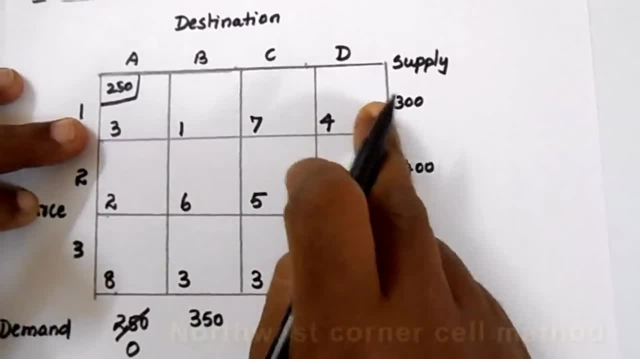 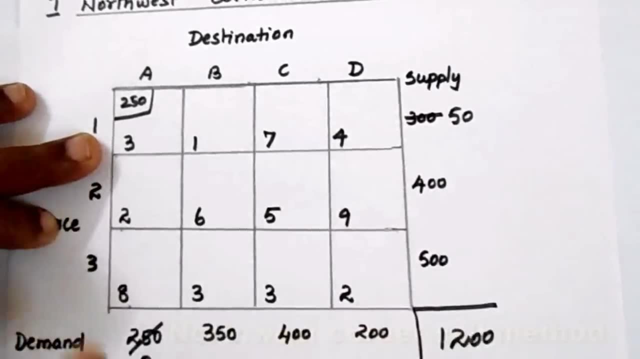 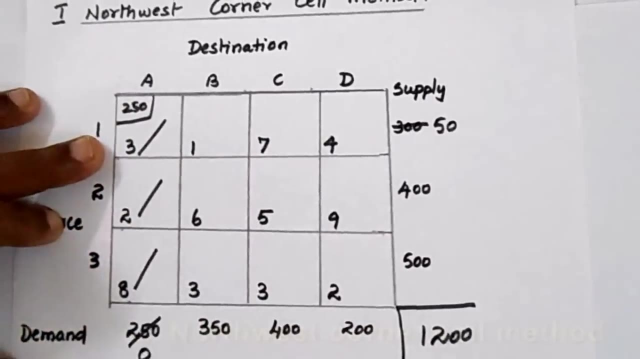 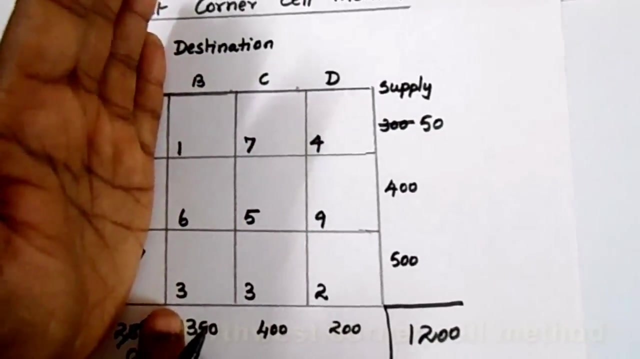 just cancel. put zero this row. 300 is there. we have allocated 250. 250 demand met remaining 50 supply is there. so this column we got zero. no, so the entire row will be get cancelled. after deleting first column, the remaining cell is like this: now we have to see which one is north, northwest corner. 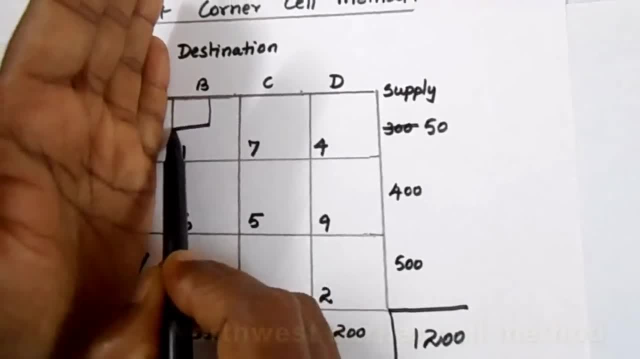 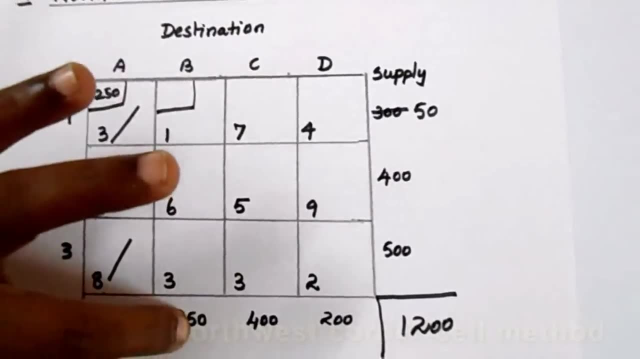 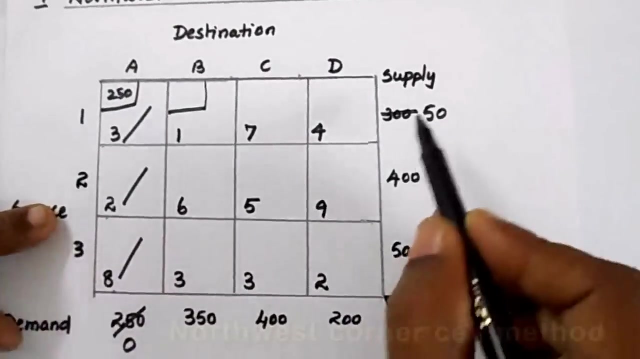 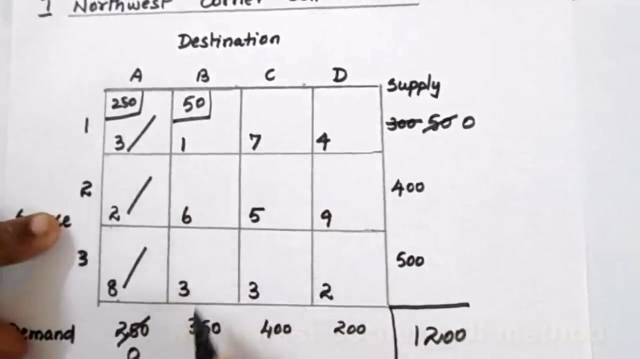 this is the northwest corner again. select this cell and see the demand and supply of respective cell for this particular cell. demand 350, supply 50, which one is lesser value, supply is lesser than the demand. so allocate 50 rupees 50. cancel will get zero. for this 350 is there no 50 match remaining 300. 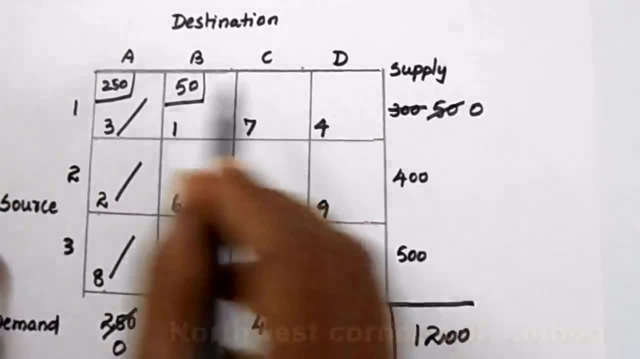 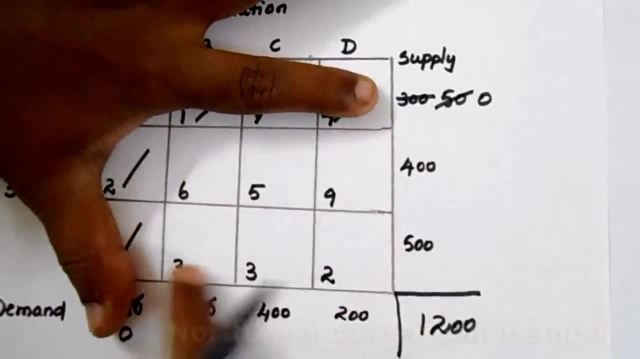 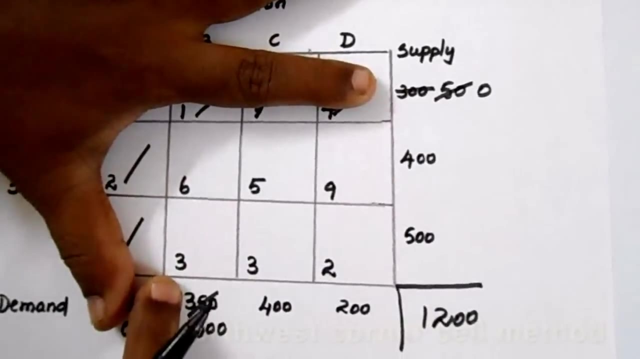 demand is there for this row. we got zero. no, the entire row will get cancelled. So, after deleting the two things, this is the remaining cell. remaining figure: unallocated cell. Out of the unallocated cell, find the north west corner. Which one is north west corner? This is the north west corner cell, So start. 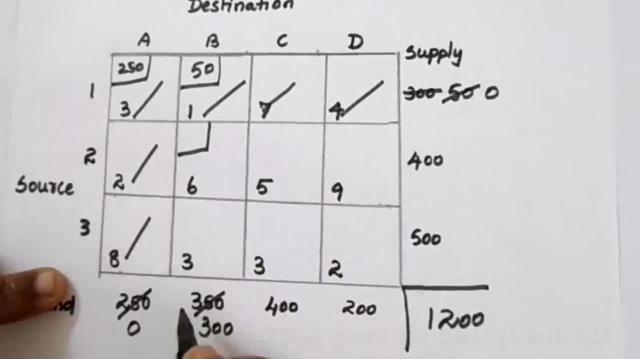 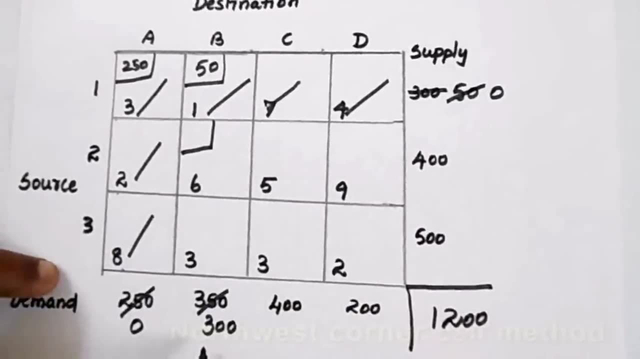 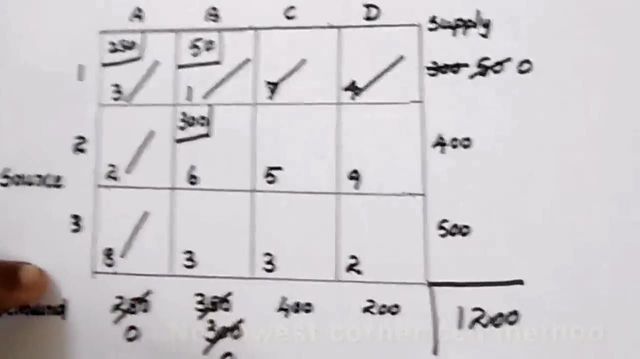 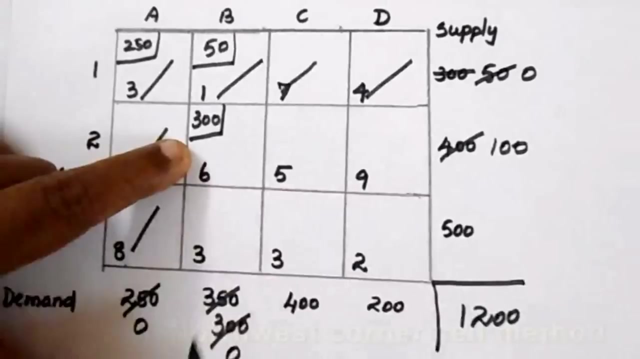 allocate For this column: 300 demand is there. For this row: 400 supply is there. Which one is less? Demand is lesser than supply. Put 300 here, Just cancel 0, because 300 is allocated. 400 supply is there, 300 is allocated. We will have only 100 rupees Here. we got 0 now. 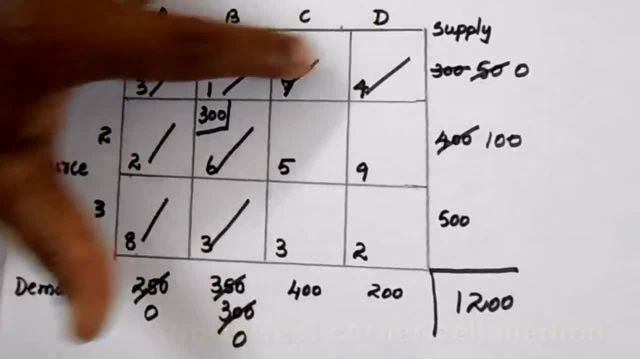 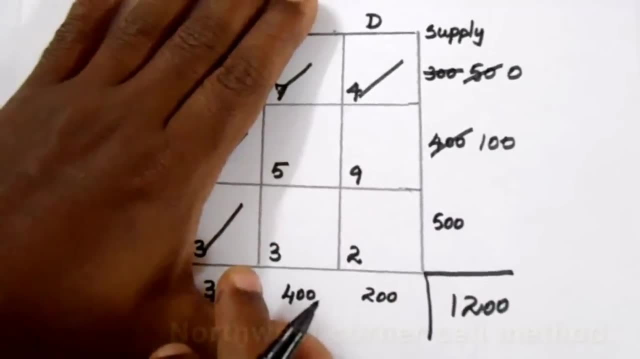 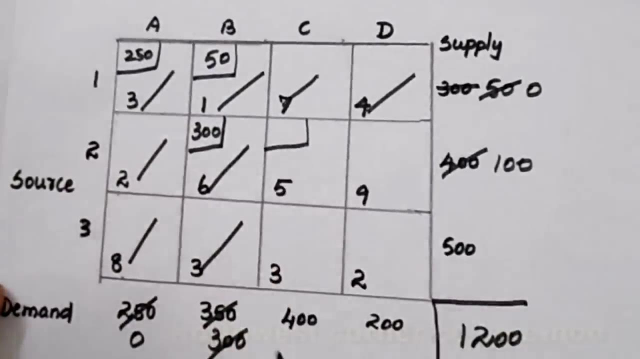 Just cancel this column. After deleting all these things, this is the remaining unallocated cell. With this unallocated cell, find the north west corner. This is the north west corner. So select this cell and allocate the value So which one is less? Just compare. 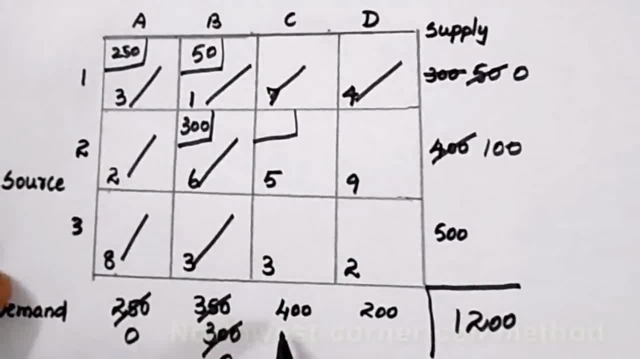 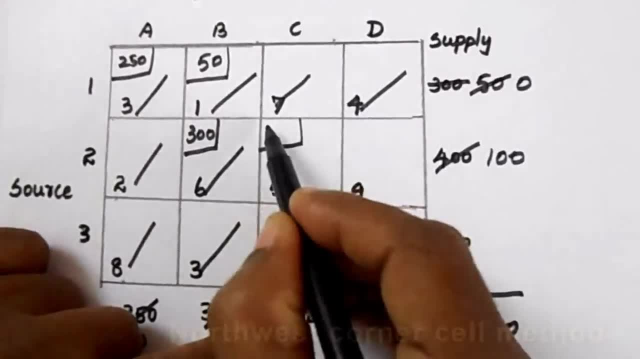 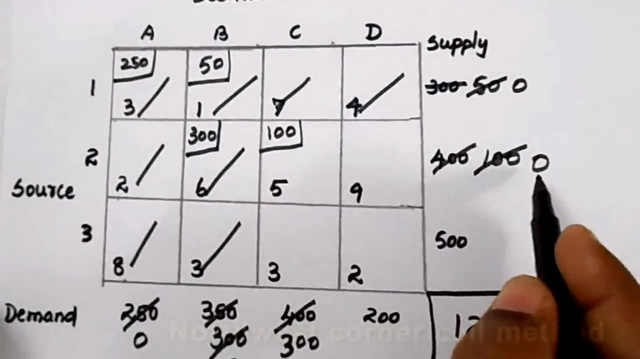 the row value and column value. Column value is 400 for this cell and row value is 100.. So which one is less? 100 is less, 100 is lesser value. Just write 100 here and you will get 0 and out of 400, 0. now Just cancel this. Now we have only 2 cells. This is the north. 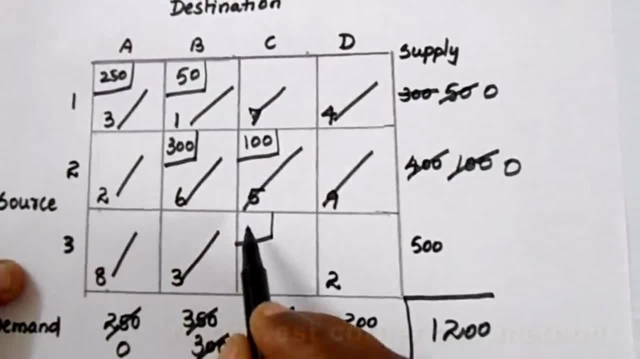 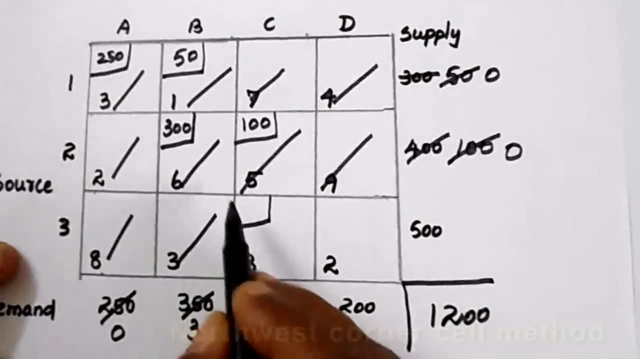 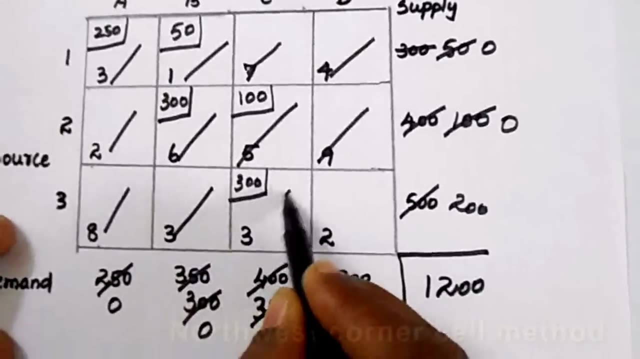 west corner. now Allocate this cell. We have got 300 demand and 500 supply. Which one is lesser value, Demand is less, So put 300 here, Balance 200.. Cancel 0. This also get cancelled And finally you will have only 1 cell unallocated In this unallocated cell. 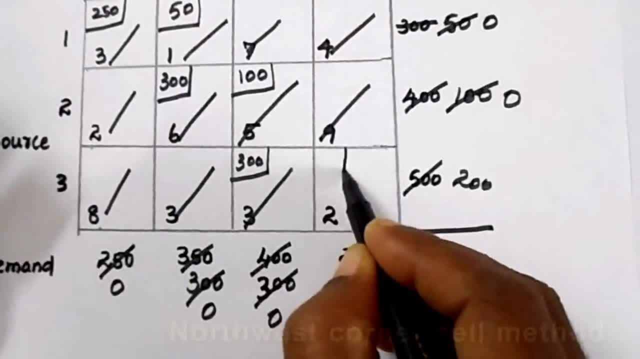 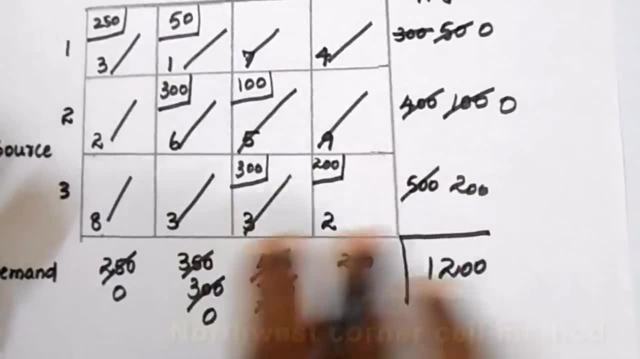 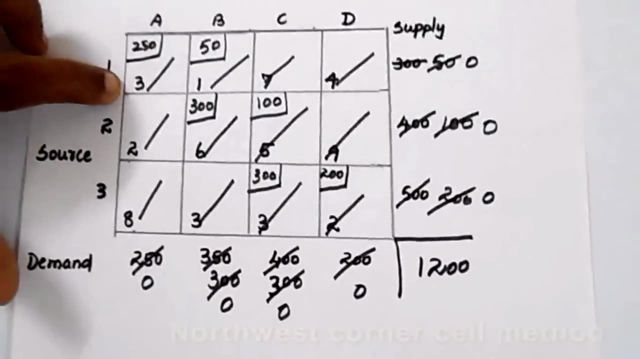 you will have demand equal to supply. Just see: demand also 200.. Supply also 200. It is a balanced problem. You won't get any balancing figure. Everything is cancelled Now. just multiply the value with the cell value In first allocated cell. 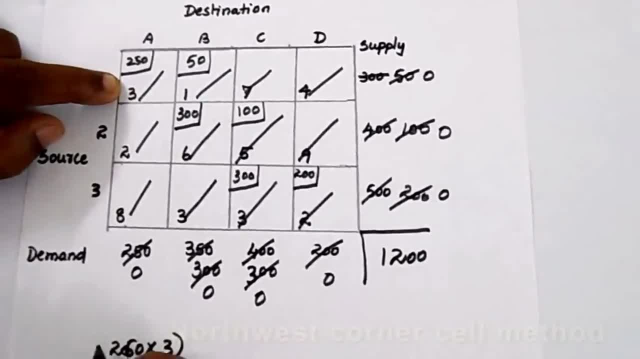 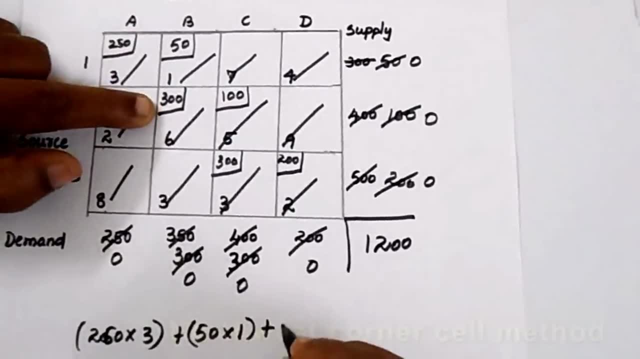 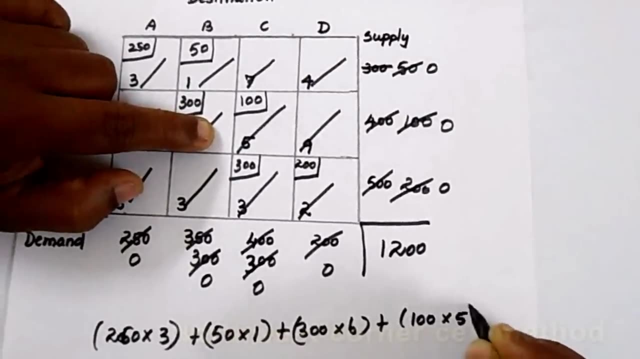 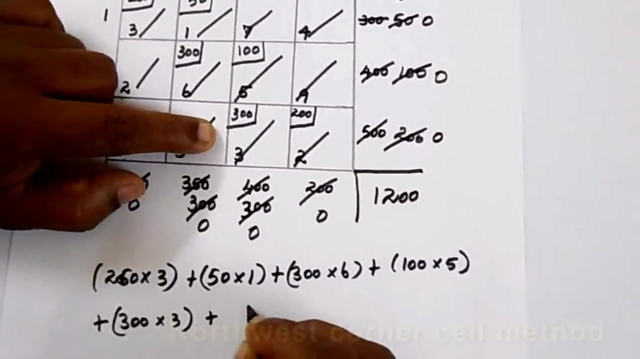 250 into 3 plus 50 into 1 plus 300, into 6 plus 50 into 1 plus 300, into 6 plus 200 into 2 plus 100, into 5 plus 300, into 3 plus 200, into 2.. Just find the value Total will. 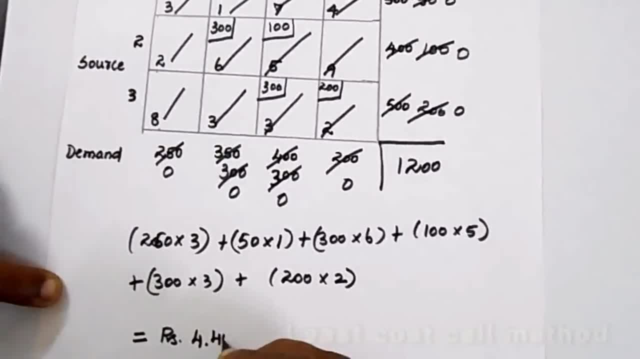 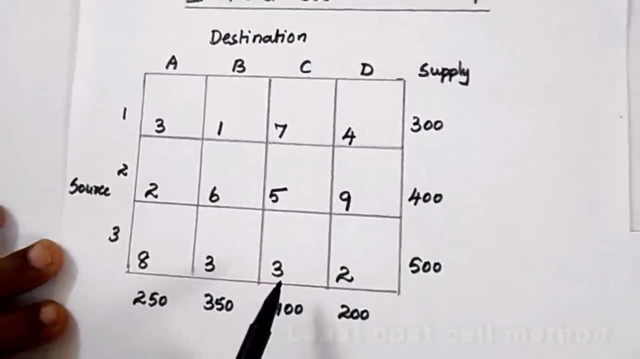 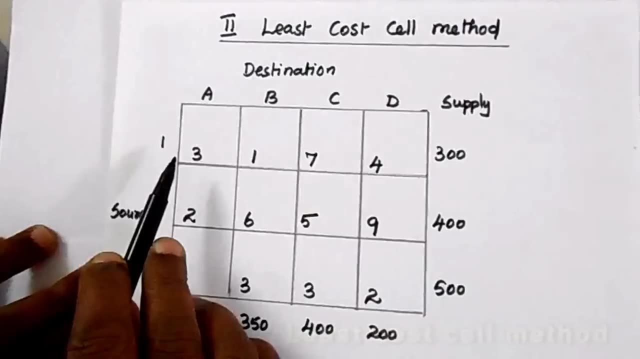 be rupees 4400.. Least cost cell method. According to this method, first we need to find out least cost among the various cells. So we have to find out least cost among the various cells. We have different sources and different destinations In each cell. we have got some. 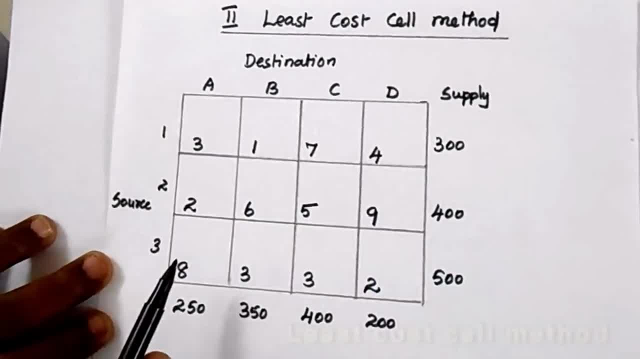 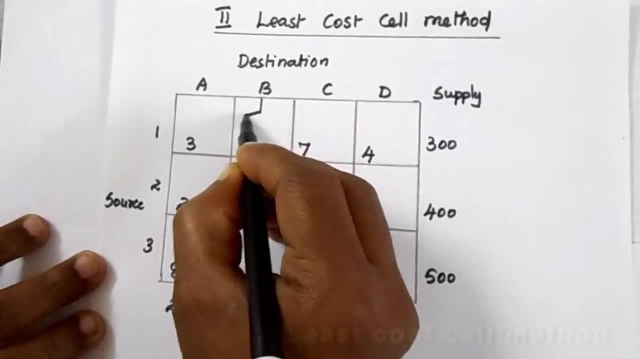 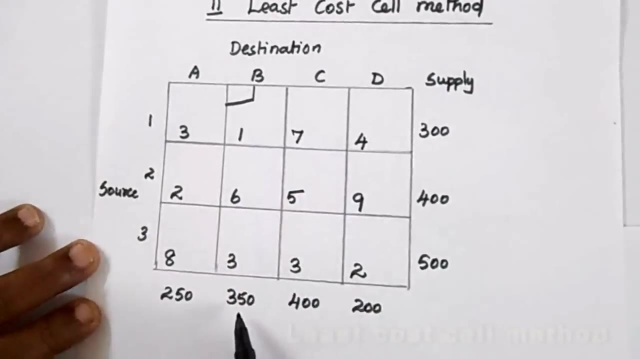 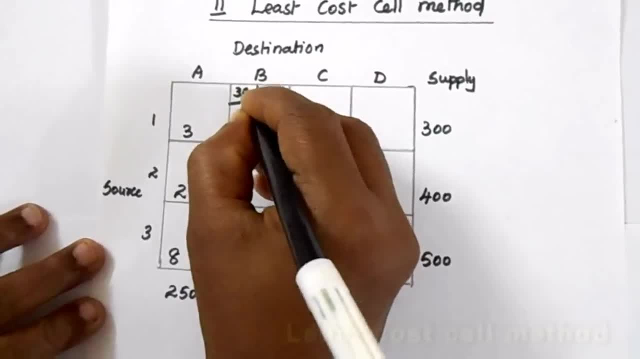 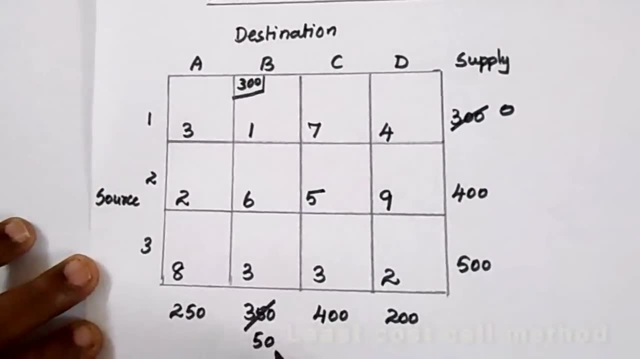 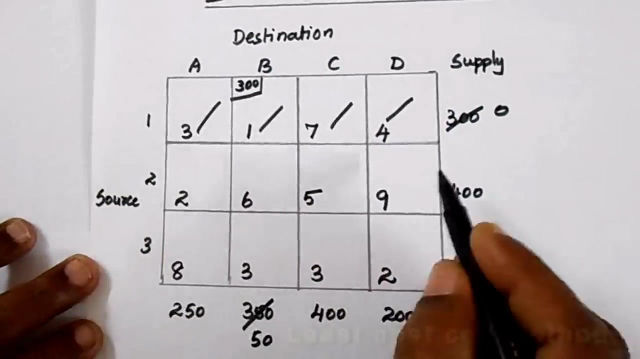 value, Demand 350 for this particular cell and supply 300.. So which one is lesser value? Supply is lesser than demand, So allocate 300 rupees, Get cancelled 0.. 350 allocated, Remaining 50. demand is there. This is 0. no, Just cancel the entire row. This is the remaining cell. 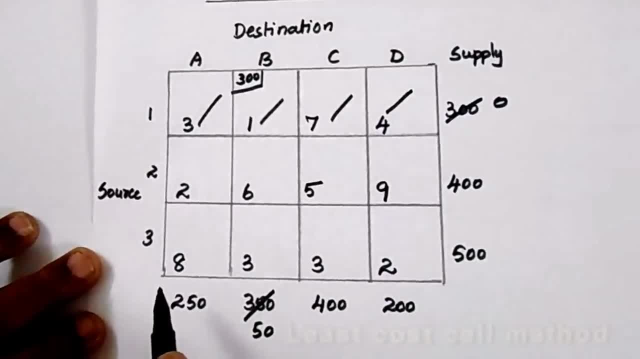 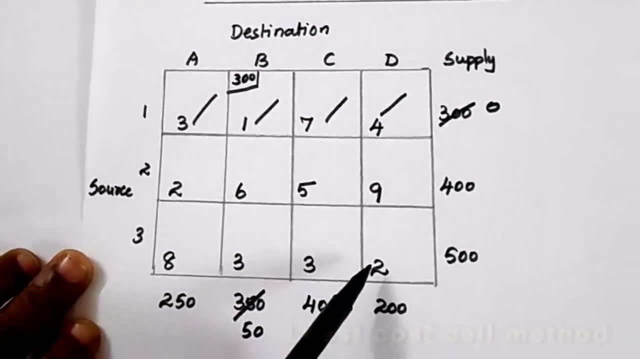 Unallocated cell Among the unallocated cell. second step is find out the least cell. You can allocate any one cell, because we have got same value in two different cell. no, So we can allocate any one. I have selected this cell. Just find out the demand and supply. 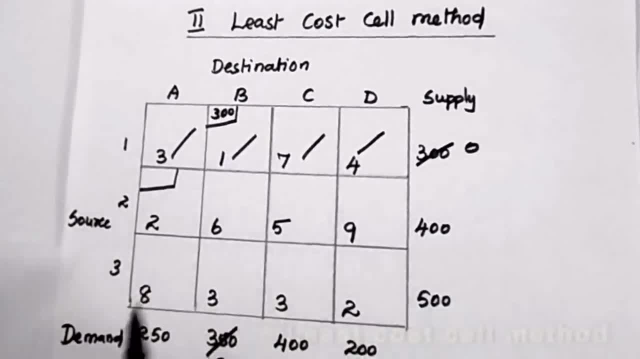 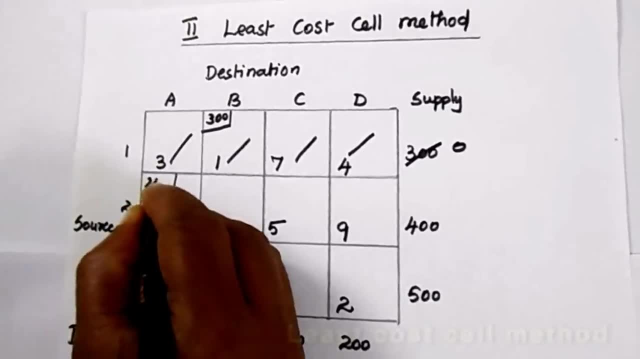 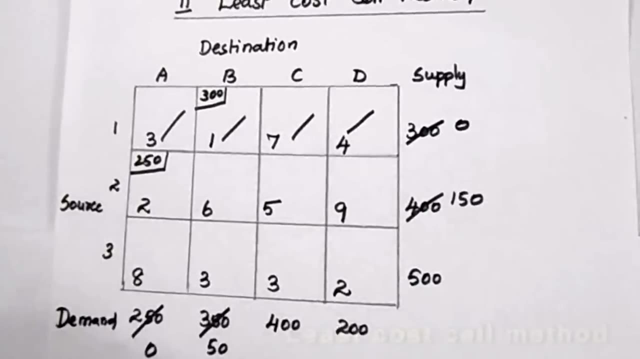 of this particular cell. So what is the demand? 250 demand, 400, supply. Which one is less? Demand is lesser than supply. Just put 250 here, 250, get cancelled 0. And here balance: 150, is there 0? no, Just cancel this column. This is the remaining unallocated cell. Now find: 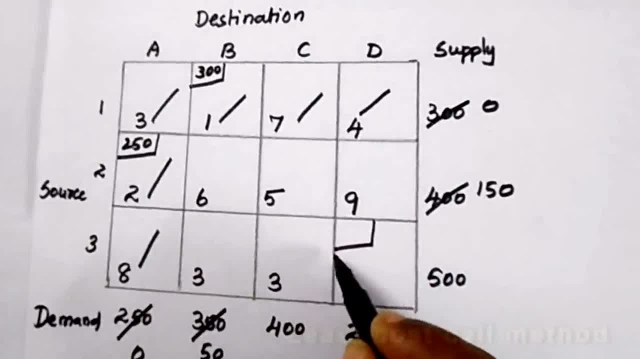 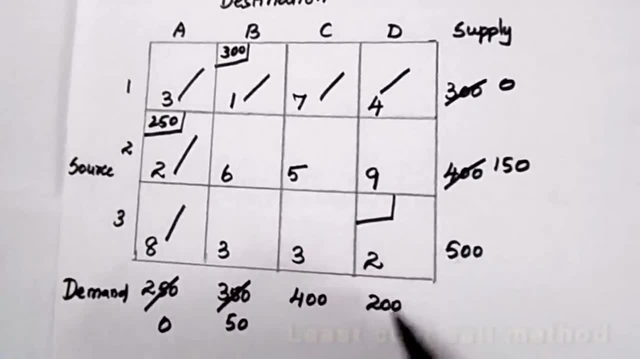 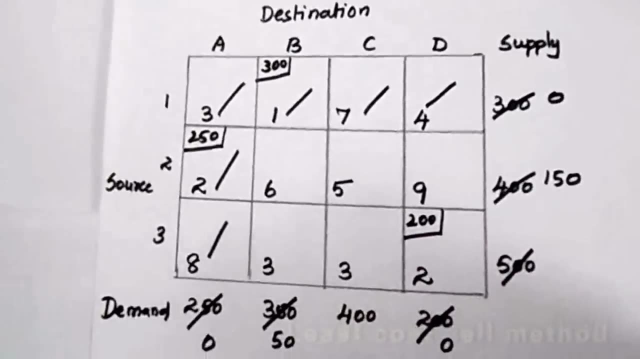 out which one is the least one among the unallocated cells. This is the least one: Demand and supply. Demand is 200 and supply is 500. So which one is lesser value? Demand is lesser than supply. So enter 200 here, 200 allocated, We will get 0. Here the balancing figure is: 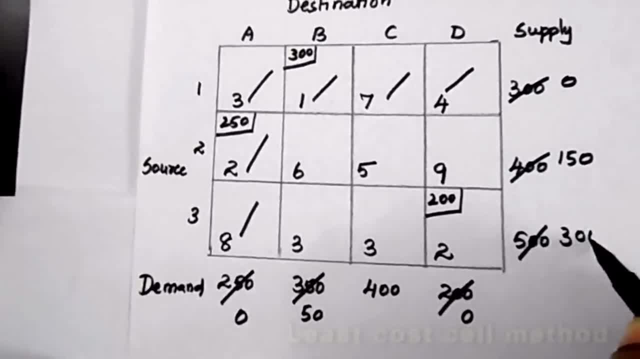 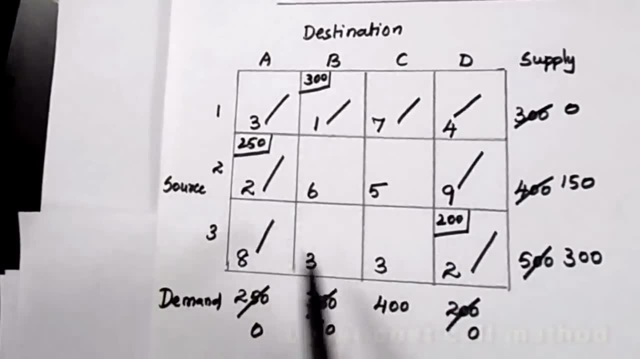 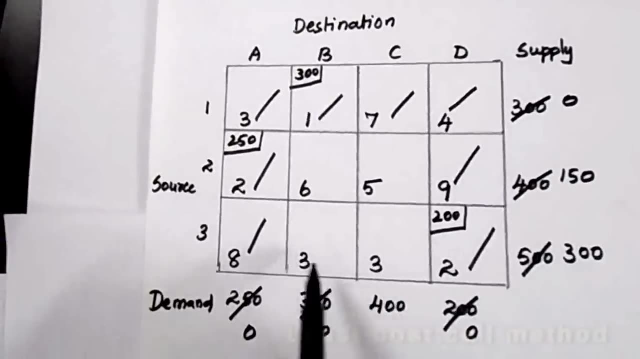 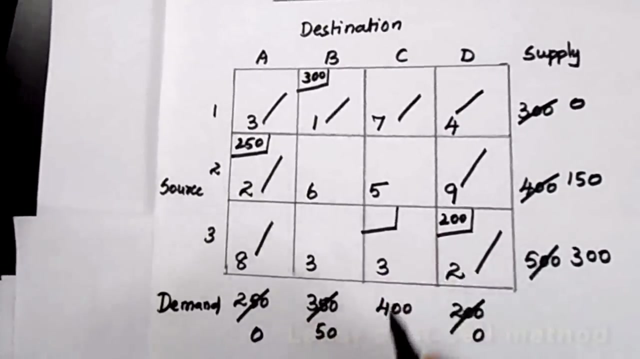 300.. This is 0. no, Just cancels this column Remaining unallocated. is there among the unallocated cells奇 least value? here we have got two, three, so you can allocate any one, just find or select this one, or you can select this also. now i'm selecting this one and find the value. demand 400, supply 300. so 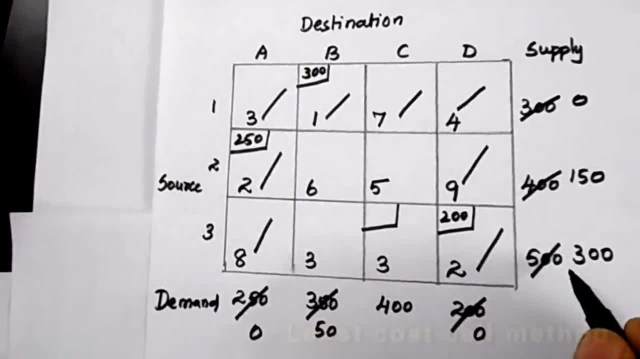 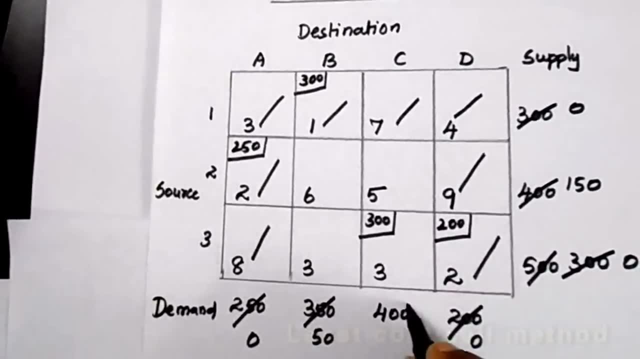 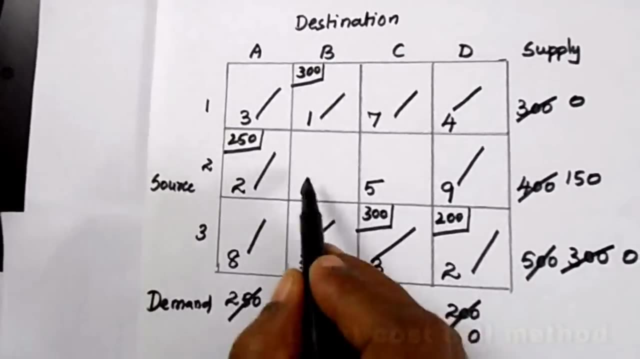 which one is lesser value? supply is lesser than demand, so enter 300, get cancelled. balance 100. so this row zero. no, just delete the entire row. now we have only two cells. which one is least value? five is least value. select this cell and allocate the value. just compare demand and supply demand. 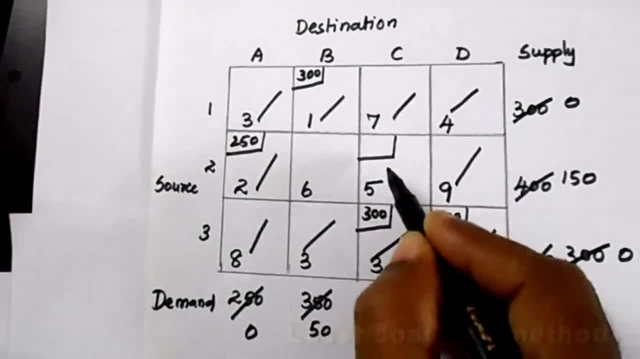 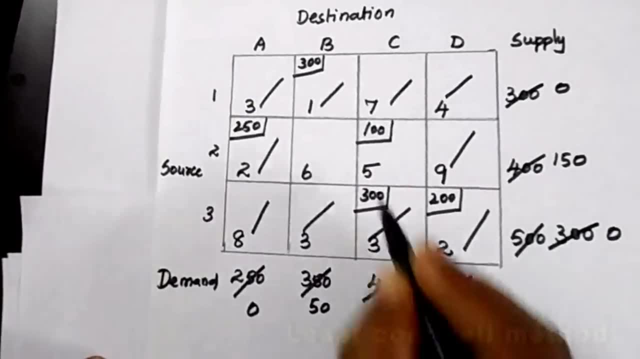 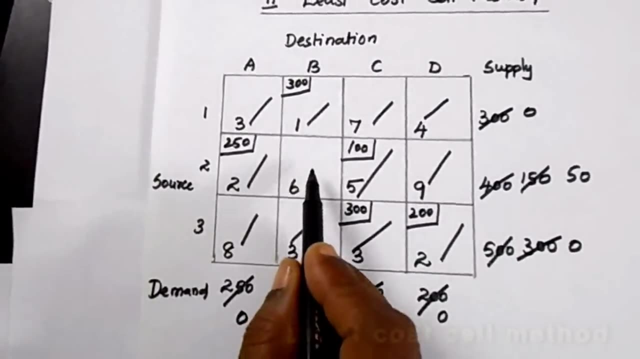 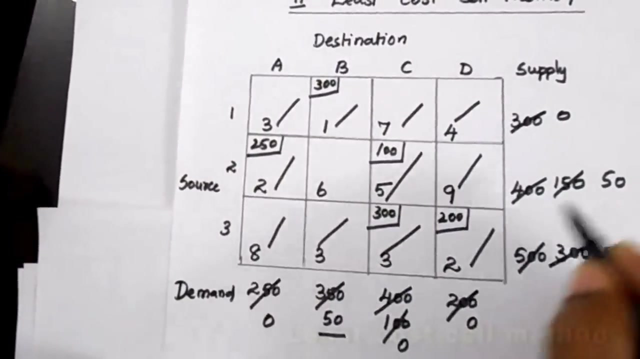 300 for this cell, supply 150. so 100 rupees is lesser than 150. so allocate 100, we'll get zero here. balancing figure: 50: zero. no, cancel this. and now we have only one unallocated cell and the balance balancing figure, that is: demand is equal to supply, demand also 50, supply also 50, just allocate 50. 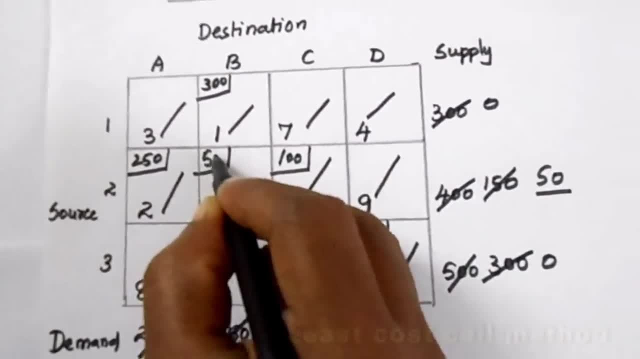 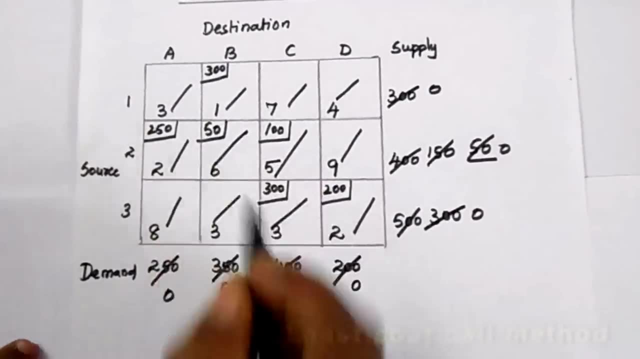 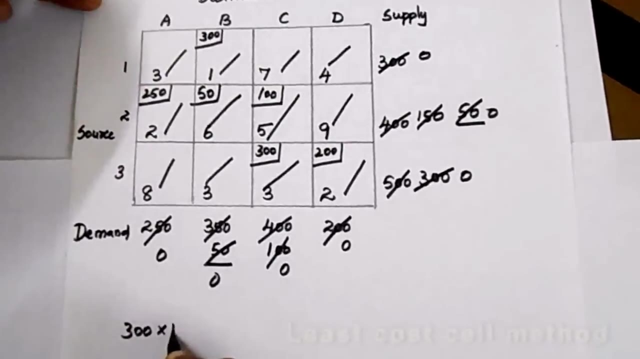 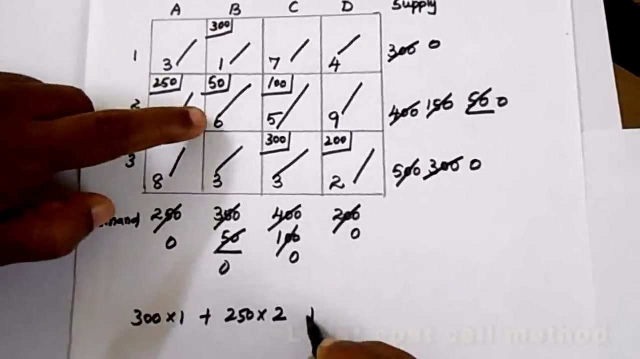 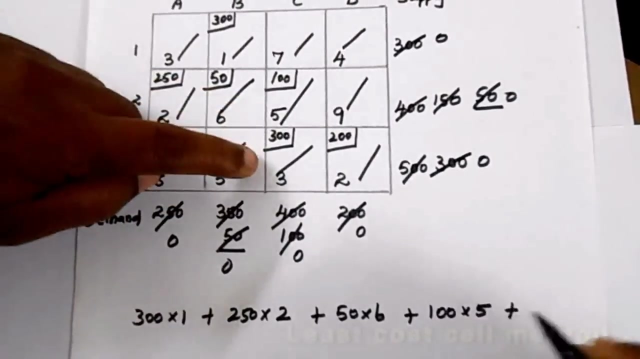 all supply and demand get cancelled. now just multiply the value and find the answer. first: one 300 into one second cell- this is the second cell- plus 250 into two, plus 50 into six, plus 100 into five, plus 300 into three, plus 200 into two. 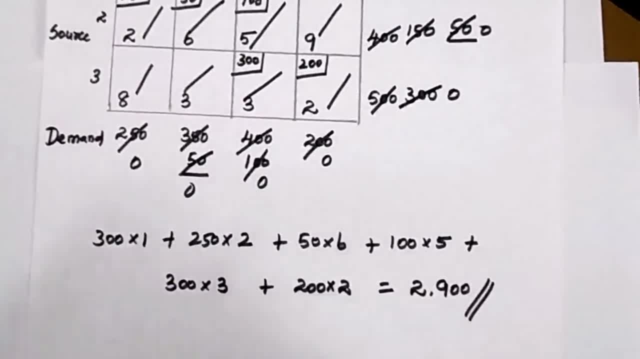 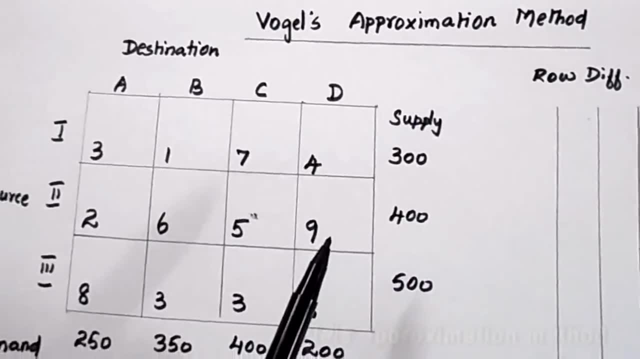 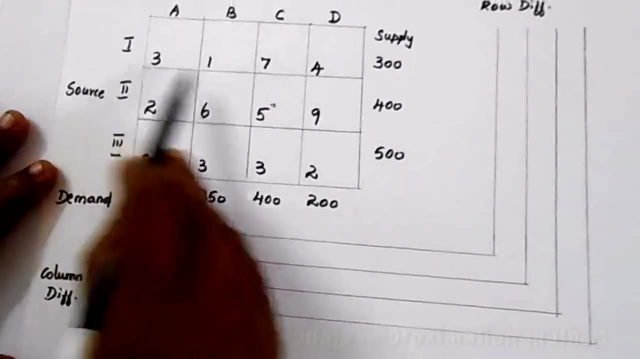 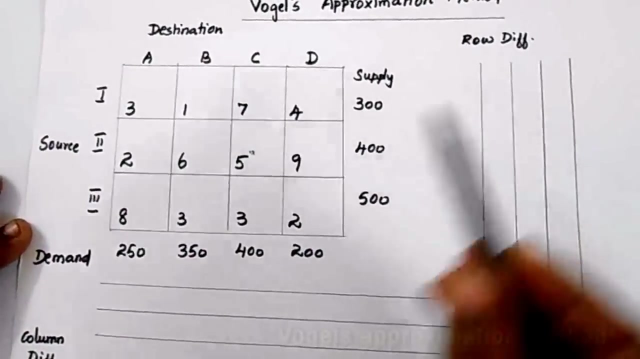 2900. okay, let us see ogle's approximation method. according to this method, before we solve the problem first we need two: find out row difference and column difference for each and every row and for each and every column. we need to identify row difference and column. 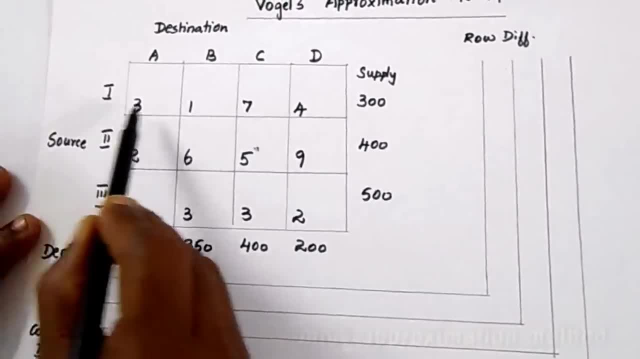 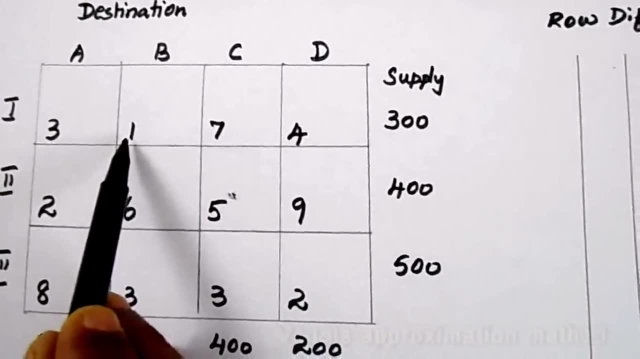 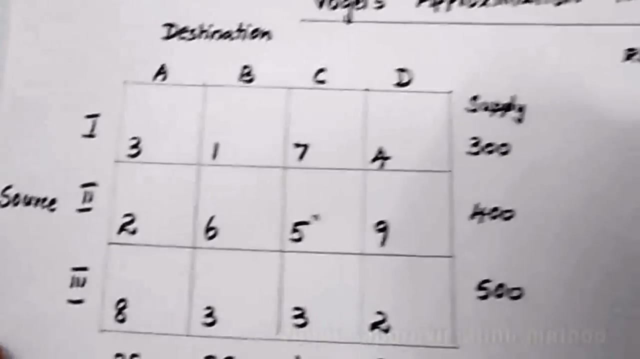 difference. how can you find out the row difference? first, select the least cell in the first row. which one is least value? one is the least value. which one is the next least value three. now find the difference between these two. least value: 3, 2. in the same way, we need to identify row difference and column. 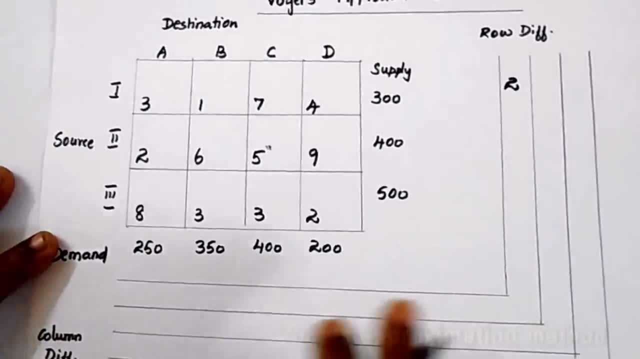 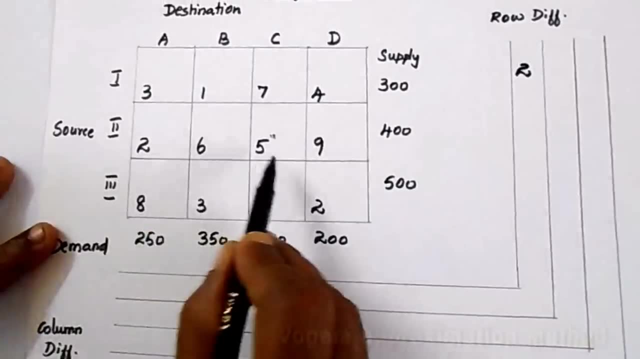 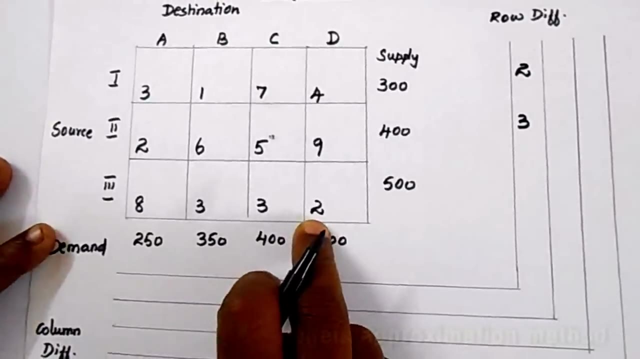 difference for each and every row, as well as each and every column. in second row, 2 is the least value, next value 5. what is the difference between these two values? 3 in the third row, 2 is the least value, next least value: 3. what is the? 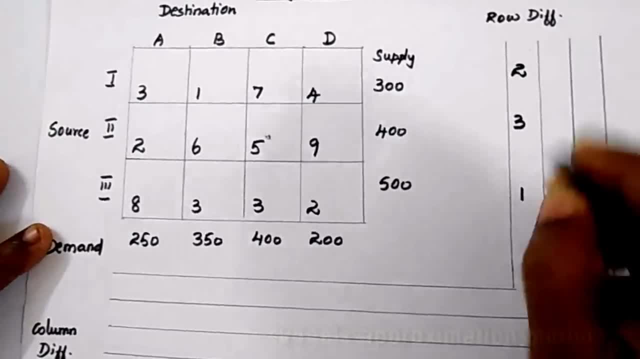 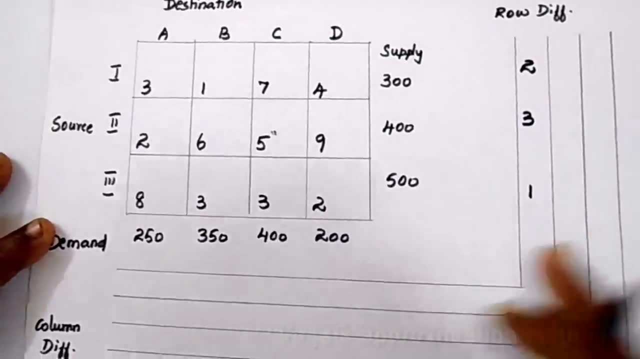 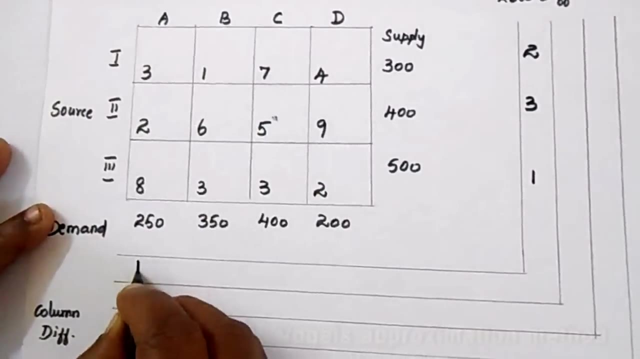 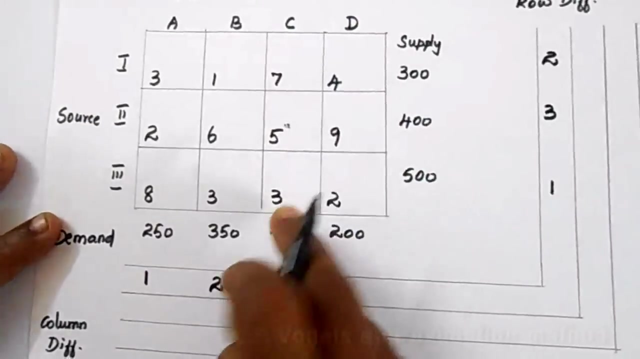 difference between these two values: 1. now, these are the row difference. in the same way, you need to identify column difference. in the first column, which is the least value, 2, next 3, what is the difference? 1 in the second column, 1, 3 difference 2 in the third column: 3, 5. 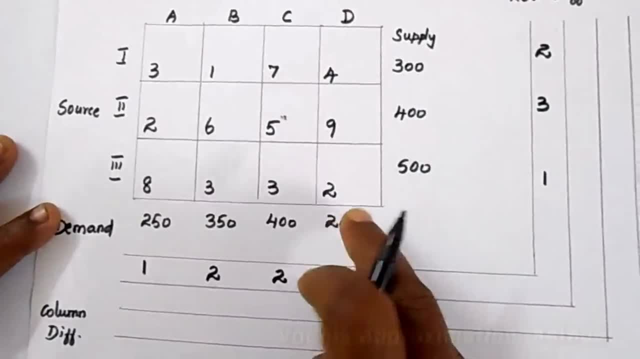 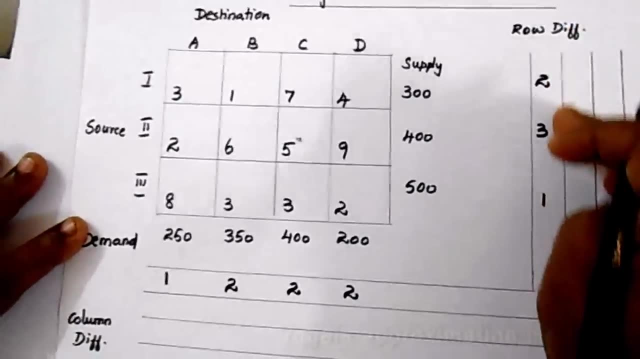 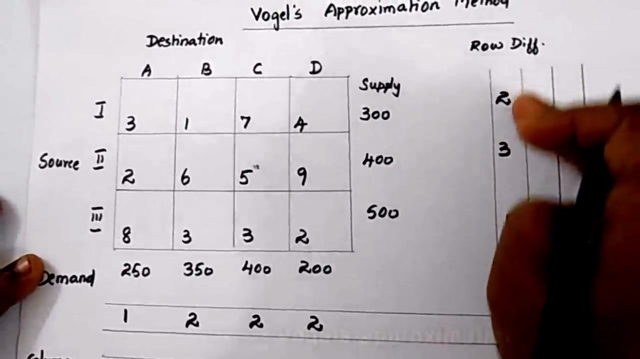 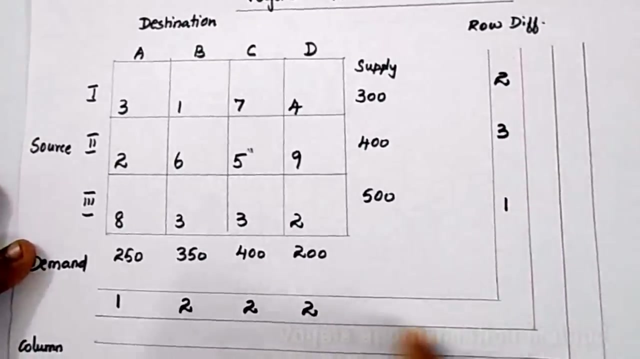 difference 2 in the fourth column. 2, least value next, for what is the difference to know? we have got row difference and column difference. then next step is select the maximum penalty. these are the values called us penalty rope, and I am drawing penalty among these value. you have to find out, or? 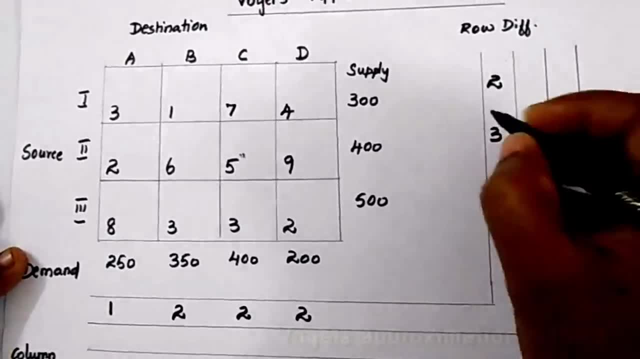 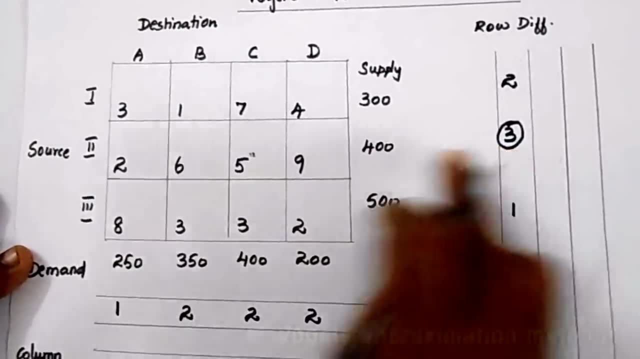 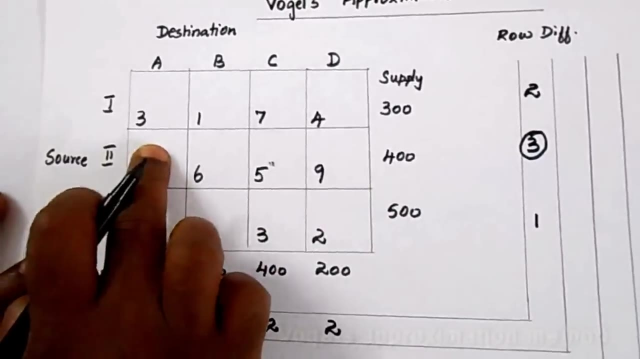 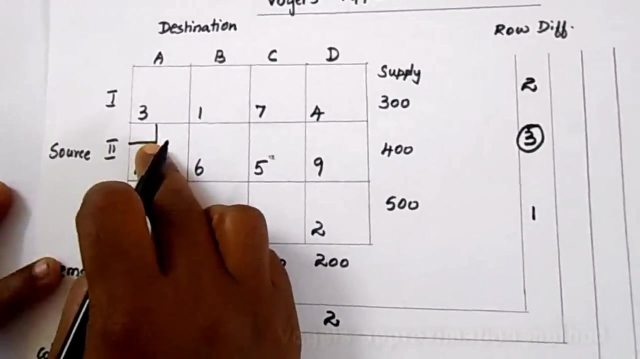 select maximum values. which is the maximum value? 3 is the maximum value. 3 occurs ain't row 2.. This value occurs in row 2.. Find the cell with the least cost in row 2.. This cell is the least value. Now, I have selected this cell. Now you need to compare demand and supply. 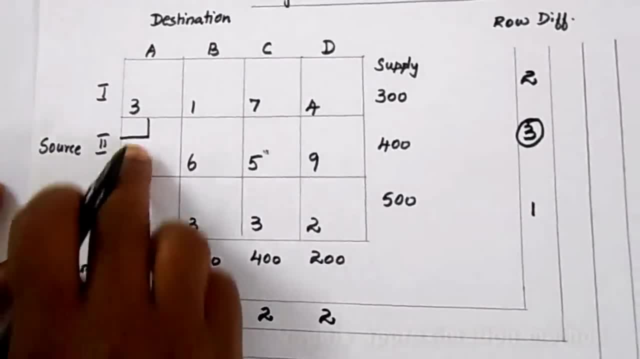 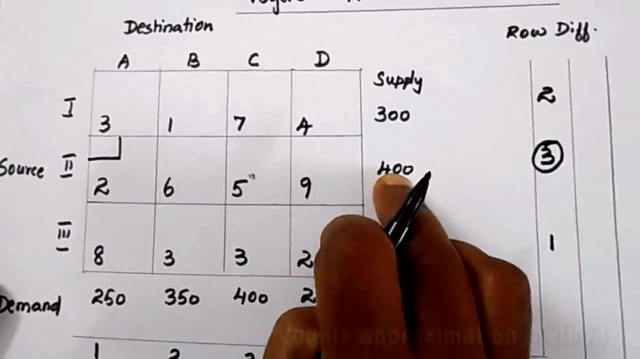 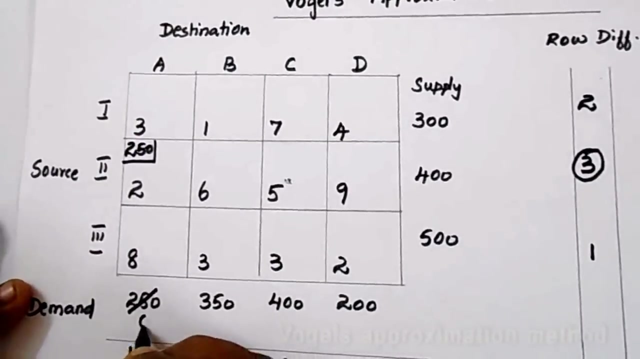 of this particular cell: Demand 250,, supply 400.. Now you have to allocate the value. So which is the least value? 250 or 400?? 250 is the least value. Just allocate 250 here And subtract this, you will get 0.. Here you will get 150.. So this row 0, no. Cancel the. 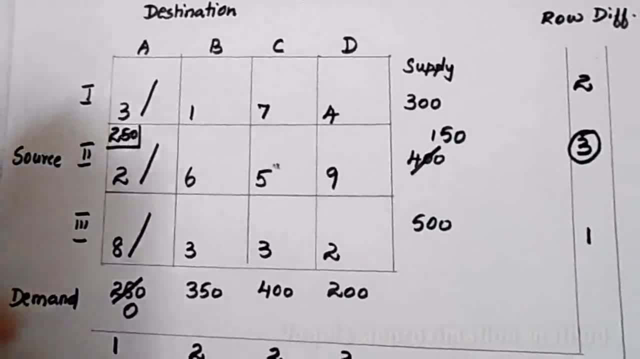 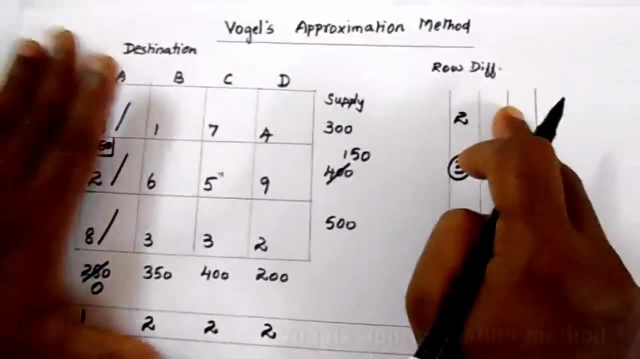 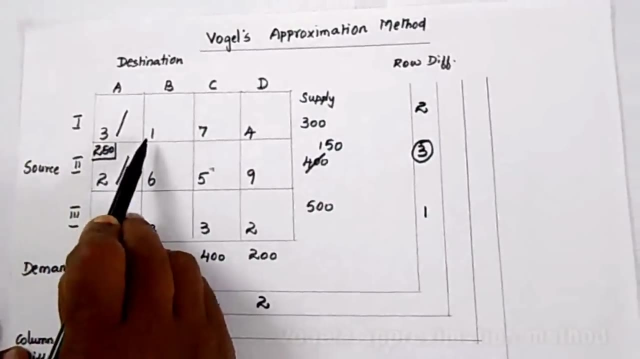 entire column. Then after this, this is the rest of the cell. unallocated cell. Again, you have to find out row difference and column difference with the unallocated cell. Again, in the first row which one is the least value, 1.. Next 4.. What is the difference? 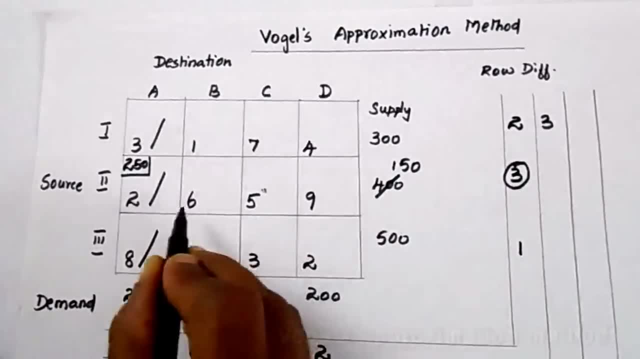 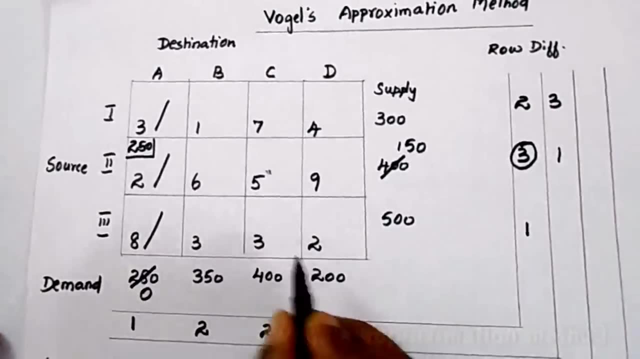 between these two values: 3.. In the second row, 5 is the least value Next value 6.. Difference 1.. In the third row, 2 is the least value Next: 3. Difference 1.. In the same way for: 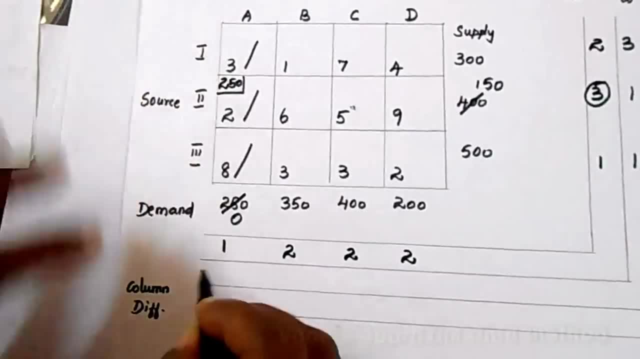 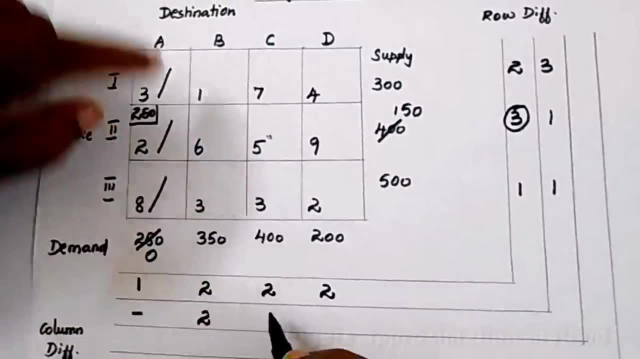 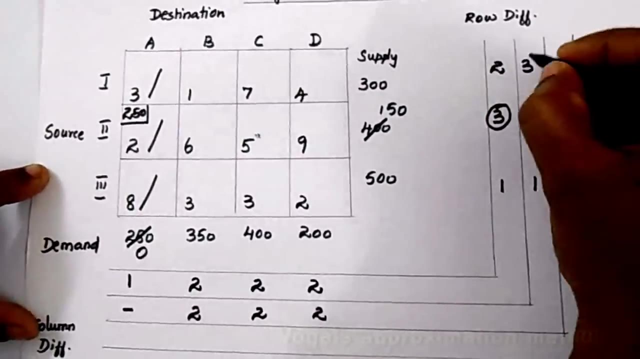 column also. So first column is deleted. Just put dash In the second column. least value: 3.. Next value: 3. Difference: 2.. Here also, 2.. Here also 2.. So among these values find out the maximum value. 3 is the maximum value, Just select. This occurs in row 1.. Again you. 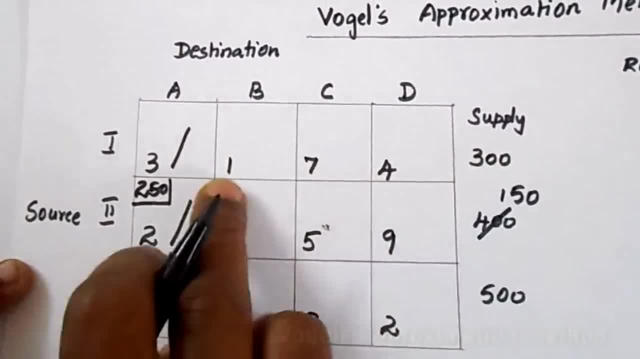 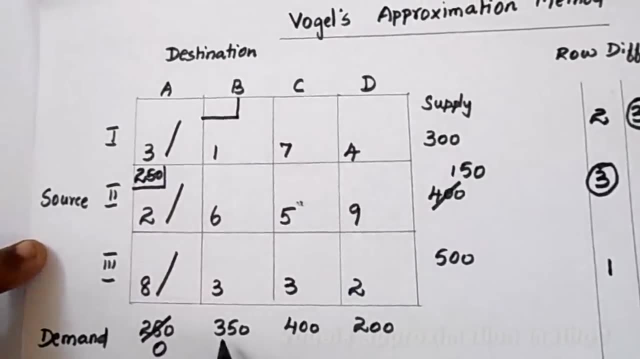 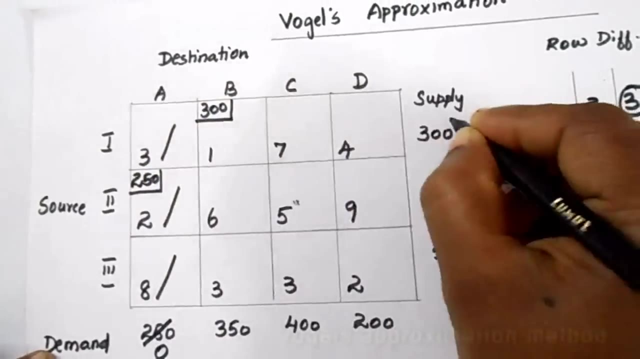 have to find out. the least cell in this first row, 1, is the least value. Just select this cell and enter either demand or supply, whichever is less. Demand: 350.. Supply 300.. Supply 300.. Take a lesser value: Just put 300. here You will get 0.. Here you will get 50 balance. 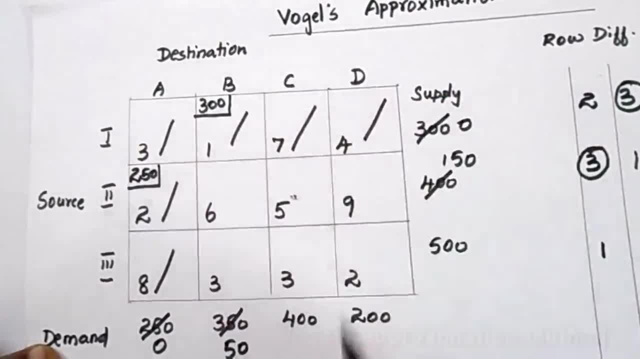 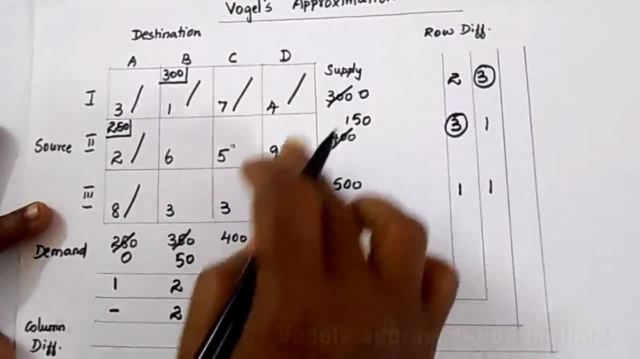 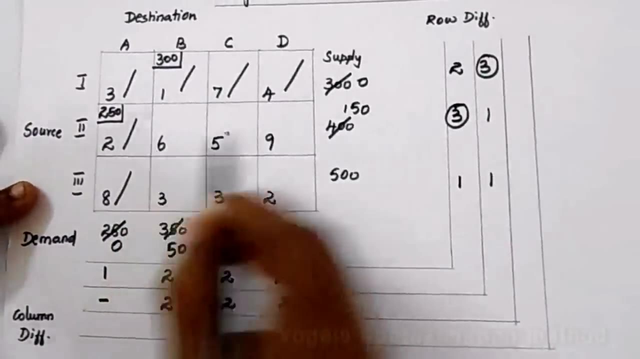 So this row got 0.. Just delete the entire row. Now. 1 row, 1 column is over. Now we have only 2 rows and 3 columns are there With this unallocated cell. again you have to find out row difference and column difference In the first row. entire thing is over, Just. 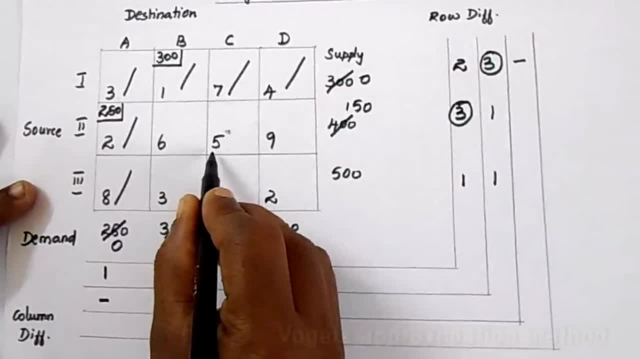 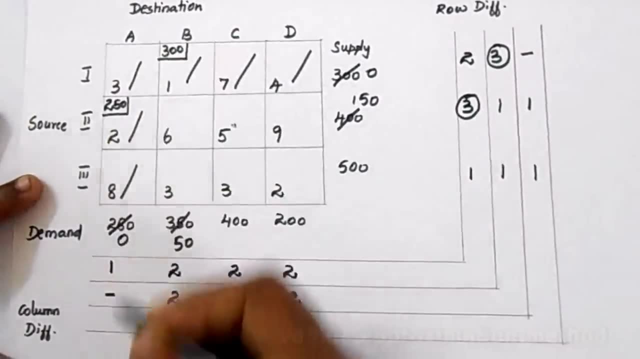 put dash In the second row. 5 is the least value. Just put dash In the second row. 5 is the least value. Just put dash In the second row. 5 is the least value. Just put next least value: 6, difference 1. here also 2, 3, 1 in the column 3: 6 difference 3, 3, 5, difference 2. 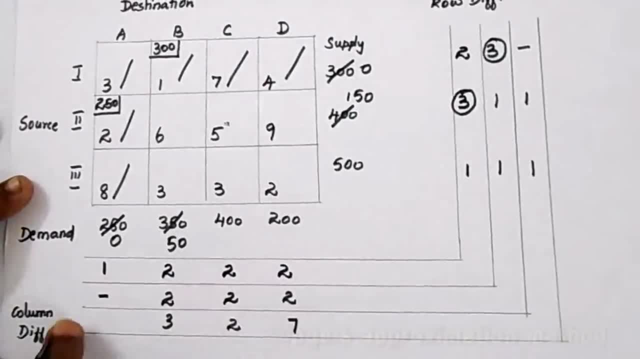 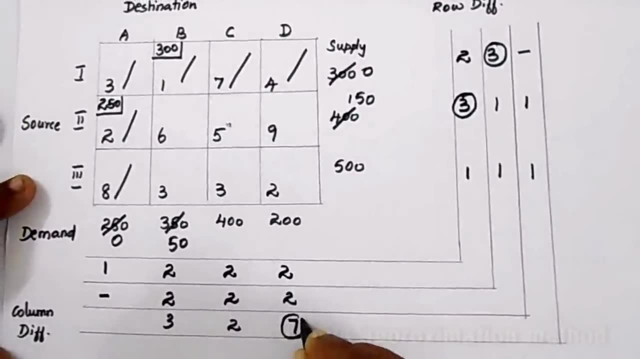 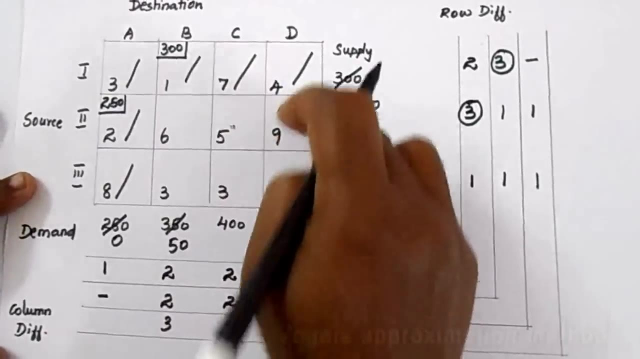 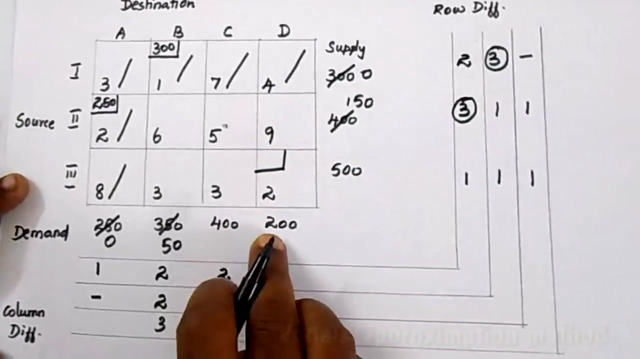 2- 9 difference, 7. among these penalties, which one is the highest value? 7 is the maximum value. just select this one. this occurs in last column, that is, fourth column among these two value, which is the least cell. this is the least cell because 9 is greater than 2. now just compare the demand. 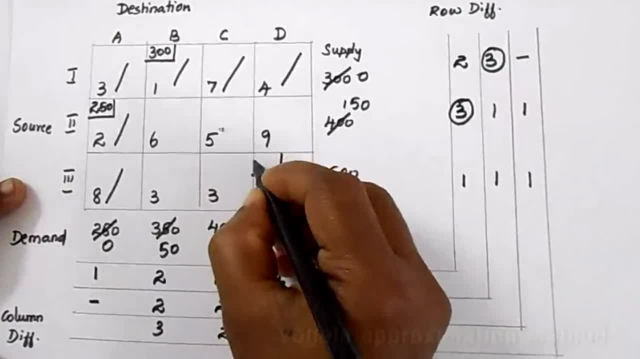 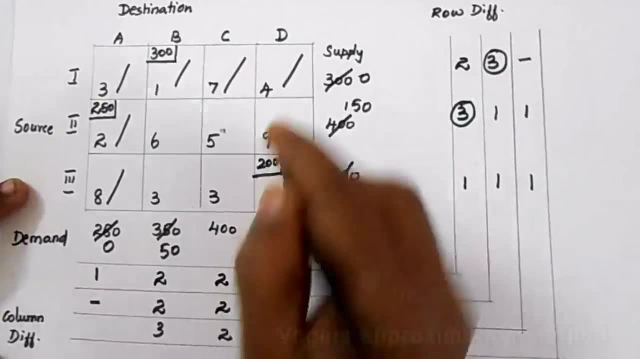 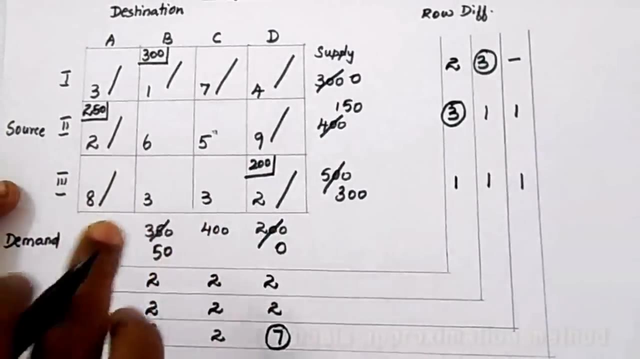 and supply. which one is lesser value? demand is lesser value. just write 200, 0, remaining 300. so this column got 0. now just delete this column. you now we have only two rows and two column. again you have to find out row difference and column. 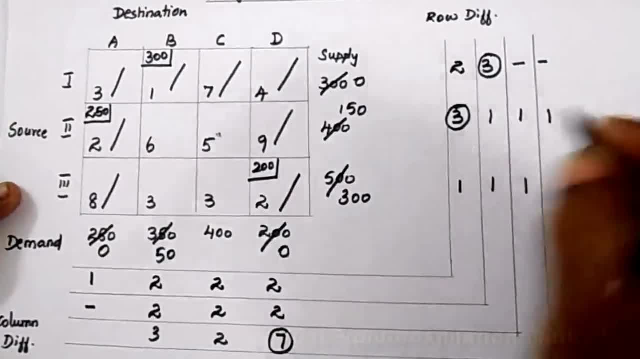 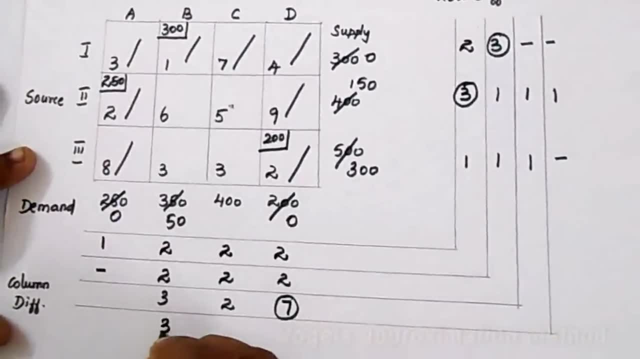 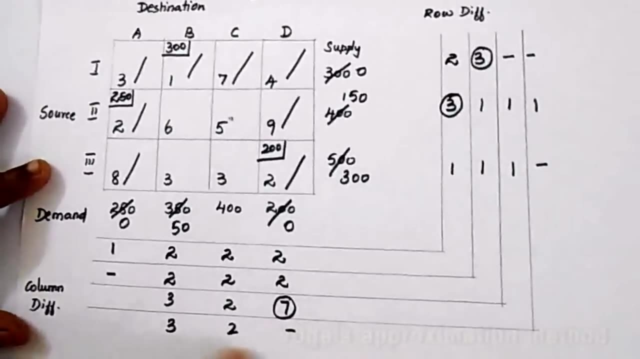 difference for this 5 and 6. difference: one for this row 3, 3, 0 and for this column 3, 6. difference for this column 3, 5, where 2 is a difference among these values, these penalties, which is the highest value, 3, it occurs. 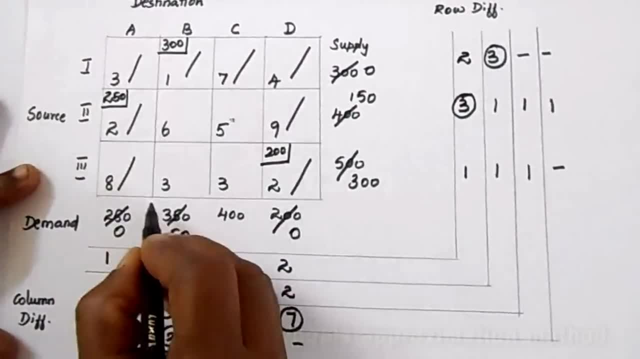 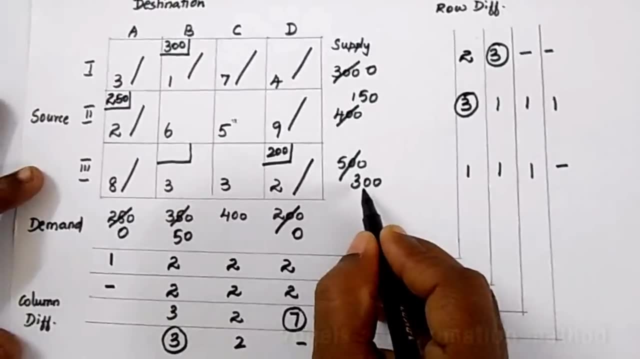 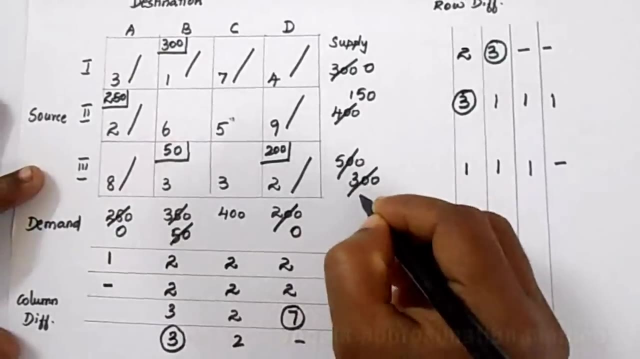 in Second column. Among the two values, which one is least? This is the least value. Select this cell, and here we have only 50, but supply 300, which is a less value. Demand is lesser value than supply. Put 50 here, Remaining 250.. Here you got 0.. Just cancel this column. 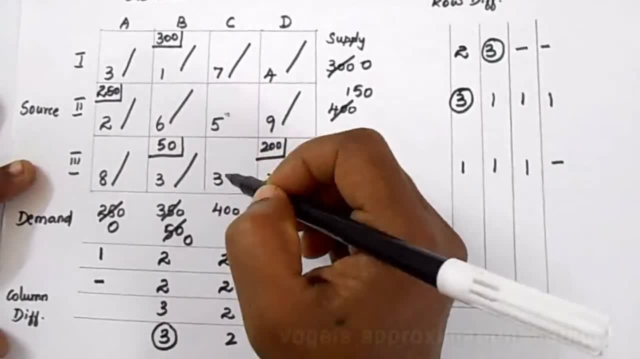 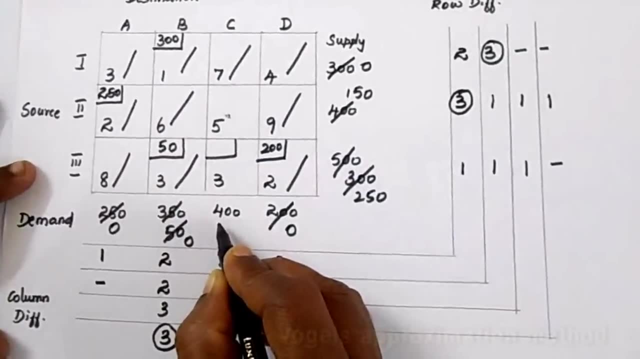 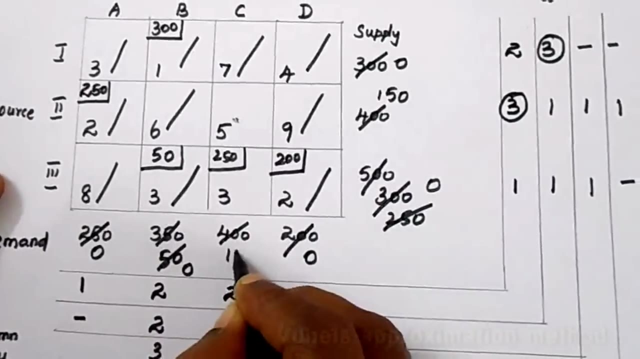 Now you have only two values. Among these two values, find out the least value. 3 is the least value. Select this cell and just see: demand 400, supply only 250.. Just allocate 250 here. Here you will get 0.. Here you will get 150.. 0, no. Cancel this row. 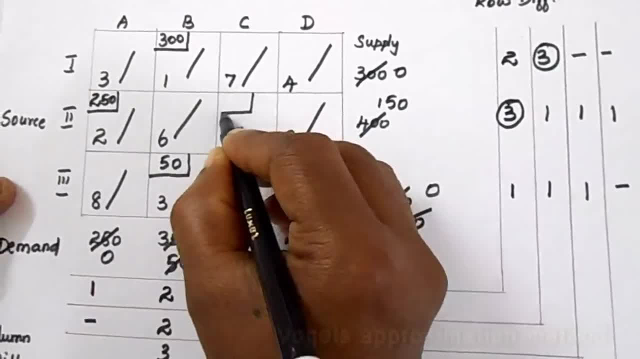 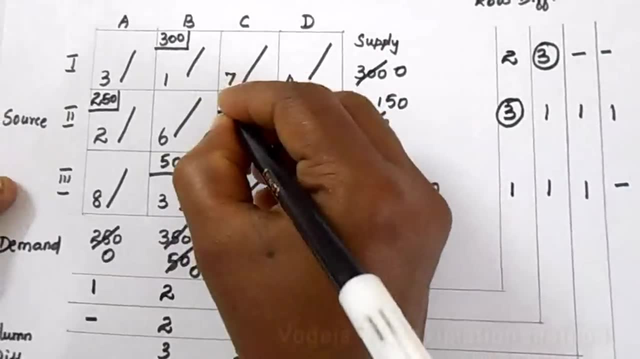 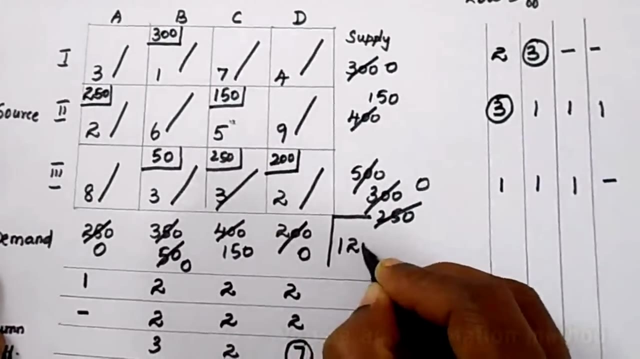 Now you have only one cell. While you have last cell, you will have equal value, Both demand and supply. And supply will be equal always. Why? Because it is a balanced transportation problem. Both demand and supply is equal. no, So the entire supply and entire demand is exhausted. 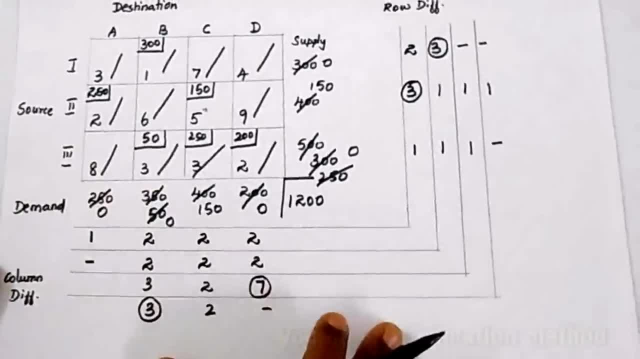 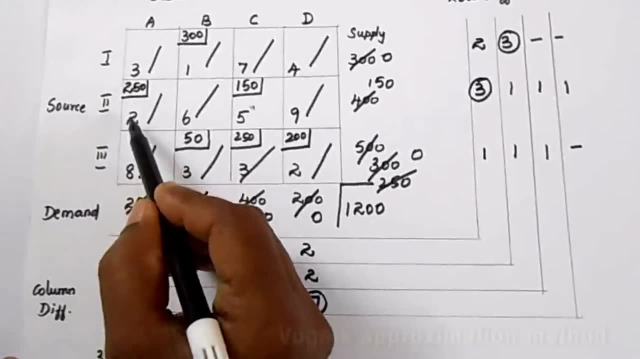 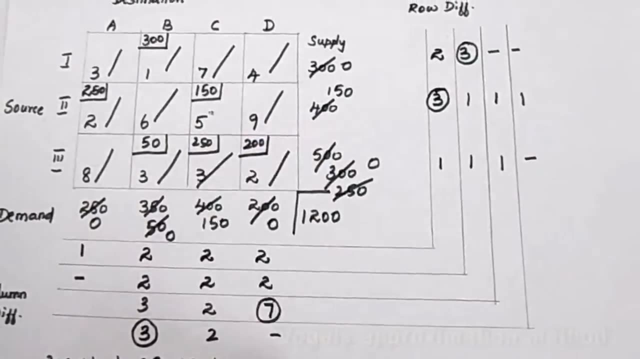 Now you can find out the total transportation cost with the allocated cell: 300 into 1.. Just multiply with the product Into 1.. 250 into 2.. Plus 1.50 into 5.. Plus 50 into 3..